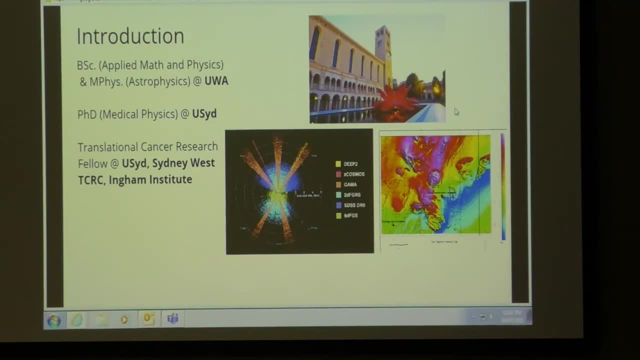 Not in medical physics- in maths and astrophysics, and then made the switch to something with a few more real world applications and moved over to Sydney and did a PhD in medical physics. I've got a varied background. I used to work in exploration: geophysics, mapping out ore reserves and things like that. 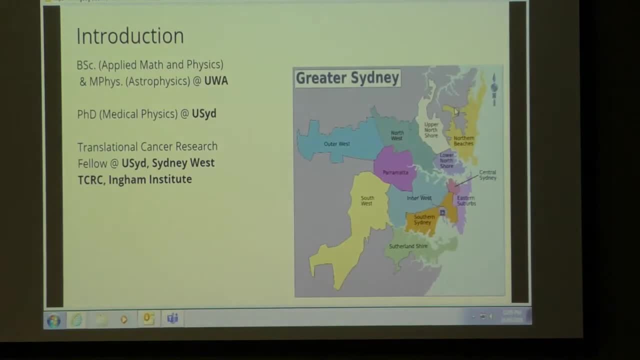 And, like I mentioned, it's some astrophysics. So in Sydney. for those of you who might not know the area so well, here's where the University of Sydney is, in the inner west, where I spend a few days a week And then I work across a few different hospitals in the metropolitan area. 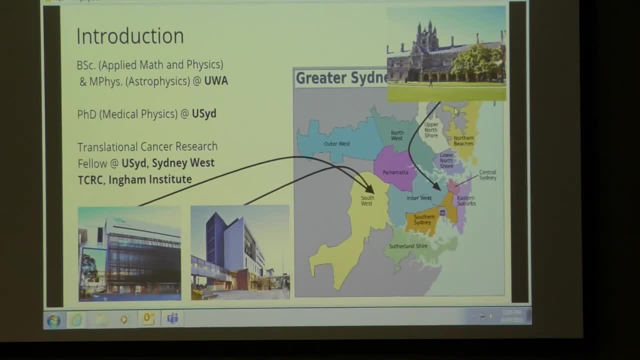 So this is where Liverpool is. It's one of the biggest hospitals and has a huge local health district, And right across the road from Liverpool Hospital is the Ingham Institute for Applied Medical Research, And there's heaps of different projects going on there, and I work in the medical physics team. 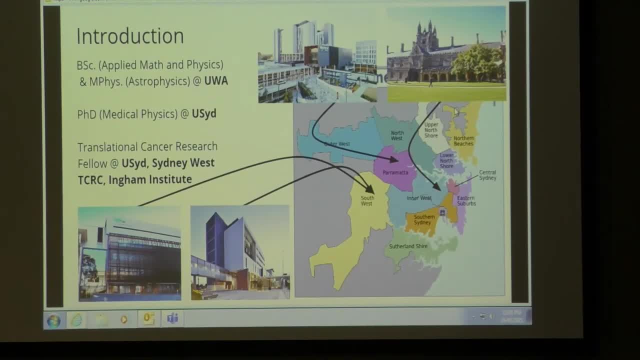 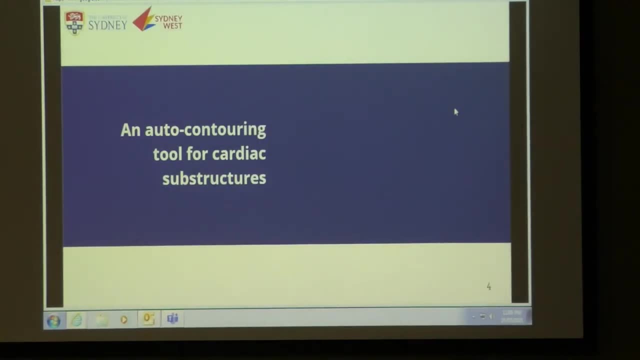 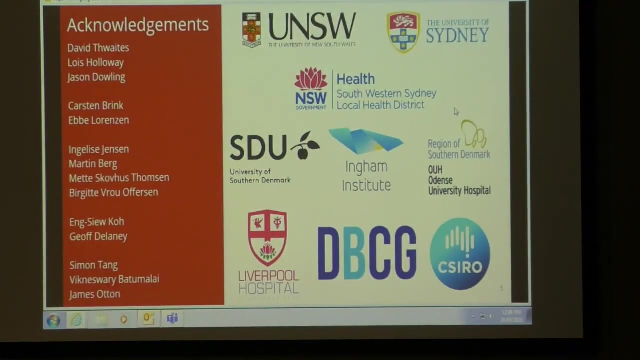 I also do a lot of work at Westmead Hospital which is up here in Parramatta. Alright, so on to the first project, which is the autocontouring tool for cardiac substructures. So of course you know, a multidisciplinary effort in making this research possible. 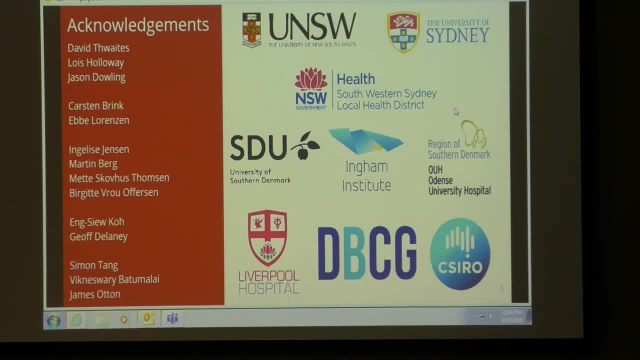 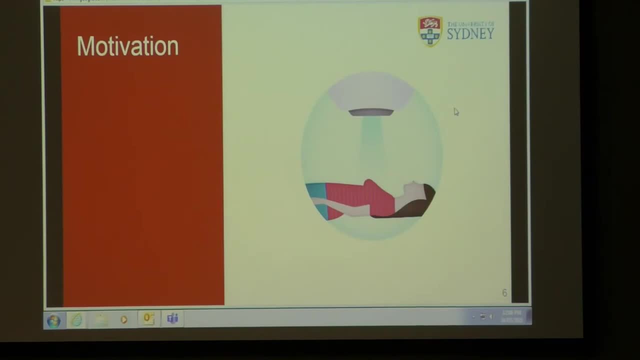 And it's supported by a lot of fantastic institutes across Australia and also internationally. So we all know that radiotherapy is an excellent treatment option for many patients with breast cancer. But there are unavoidable risks, And one of the risks that's becoming more apparent in recent years is the risk of cardio toxicities due to incidental exposure to the heart. 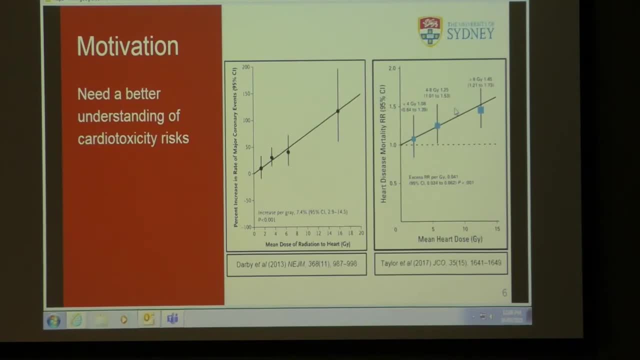 As well as breast cancer, it's also a big issue in lung cancer. So there's well-established relationships. There's a relationship between increasing dose to the heart and an increase in the risk of coronary events. This is seminal work by Darby. 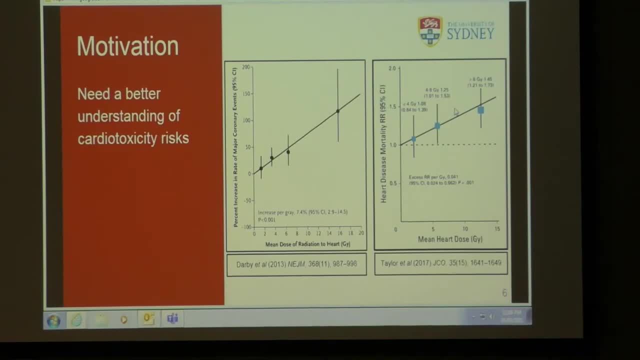 As well as overall cardiac mortality. The relationship isn't particularly well understood And it's becoming more and more apparent that using the whole heart and mean heart dose isn't really sufficient to accurately characterise the risk. You know the heart's a very complex organ. And with modern treatments we have very steep dose margins Around our organs at risk, And so you can still get very high doses to the heart in a smaller localised area, Which might mean you have a small mean whole heart dose, but still a very high risk. 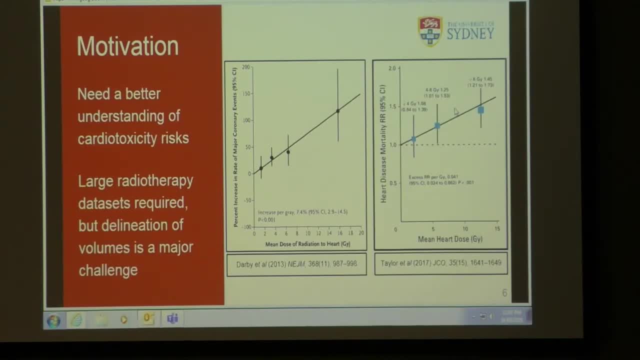 So we need to look back through our patient records, retrospective data sets, and delineate these cardiac substructures, And this poses a huge challenge. There's a lot of data to process And manual contouring isn't really a feasible option, Not only because it's so time consuming. 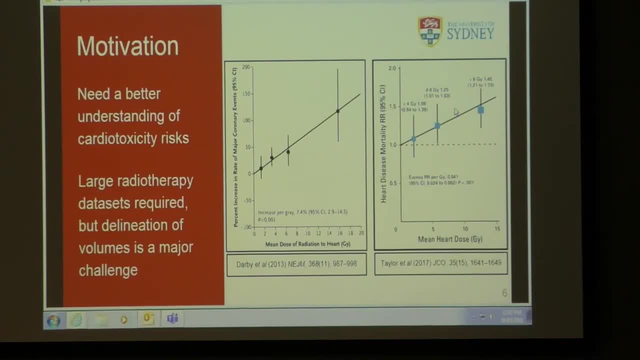 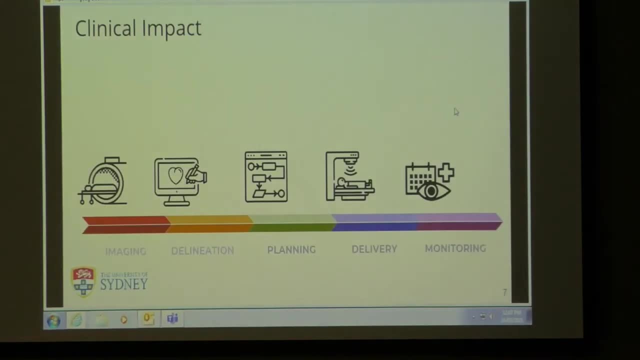 But also because there's a lot of information And we need to observe a variability that can introduce additional bias That would then affect the models that we produce. As well as this retrospective analysis, auto contouring tools are really important in the clinic. 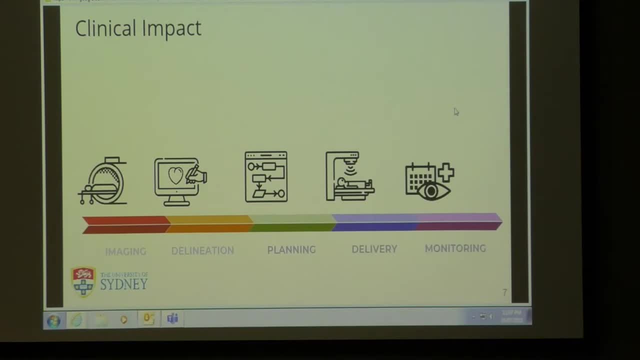 You know, moving to things like adaptive radiotherapy, for example, The amount of contouring that's required is going to only grow from here. Yeah, And there's been a few studies that have looked at delineation of target volumes And shown that that's a major source of uncertainty in the radiation therapy process. 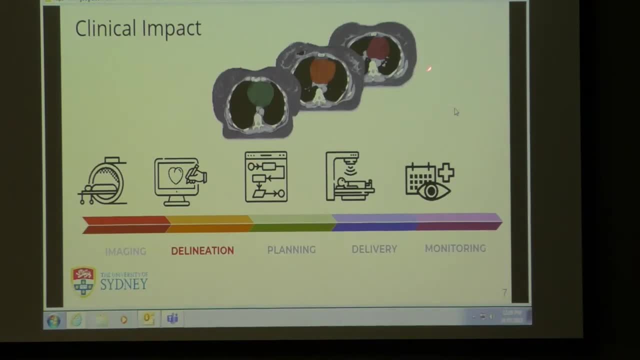 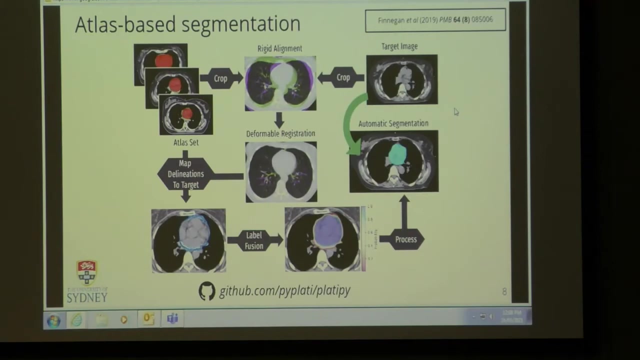 We already have huge- you know- existing data sets of patient data that's been contoured, And this gives us an opportunity to develop auto contouring models, Using AI, of course, The buzz word of the last couple of years. Alright, So the model that I set up during my PhD is an atlas based model. 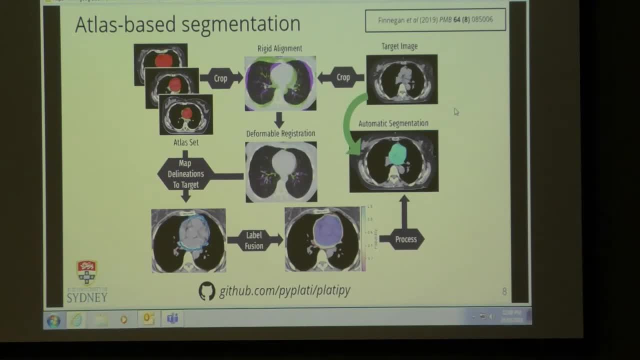 It's a little bit outdated now, But it still produces really great results, And the general idea- for those who might not be so familiar- Is that you have a set of pre-contoured patient images And you want to somehow transfer that data to a new uncontoured patient scan. 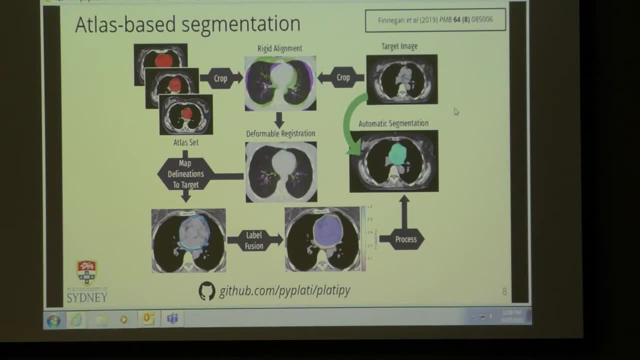 And the way that we do that is through a two step registration process. So first we align the images- So here's the target image and the atlas set. Then we use deformable image registration to define a voxel to voxel map From each image in the atlas set to the target image. 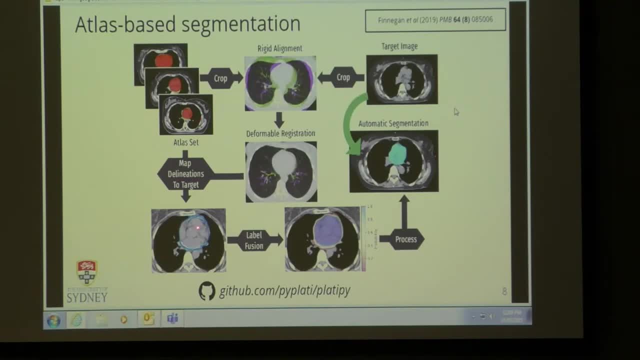 This transformation allows us to map delineations onto the target image, Where we get one estimate of the structure for each atlas. Then we use label fusion to combine them into a probabilistic label map, And I'll actually be talking about this a bit later. 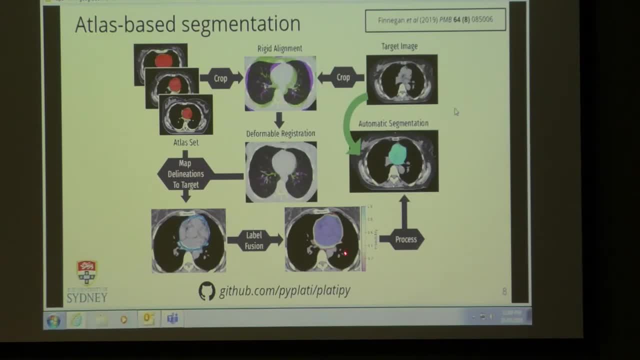 Because there's a lot of information encoded in that. Take a threshold, Get an automatic segmentation, And I'll mention now, and probably a bit throughout my talk, That all of the code is open source And available for anybody to download and use. 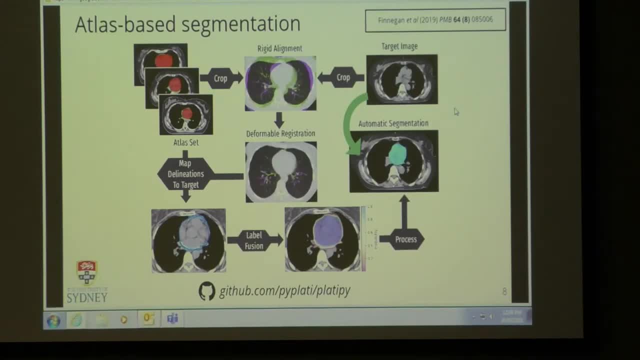 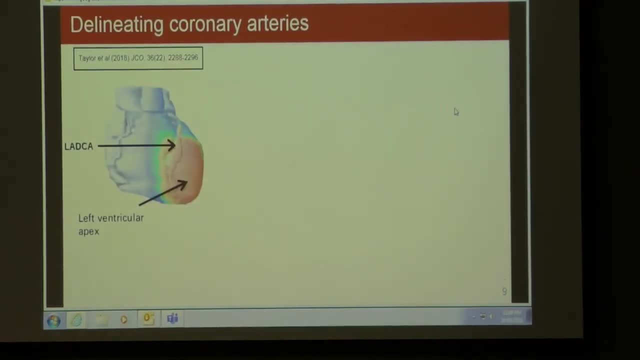 It's released under an Apache license, So you can even make commercial tools and publish them without giving me a cent. Don't do that, Okay. So one of the major challenges, though, with atlas based tools Is that they aren't very good at segmenting small structures. 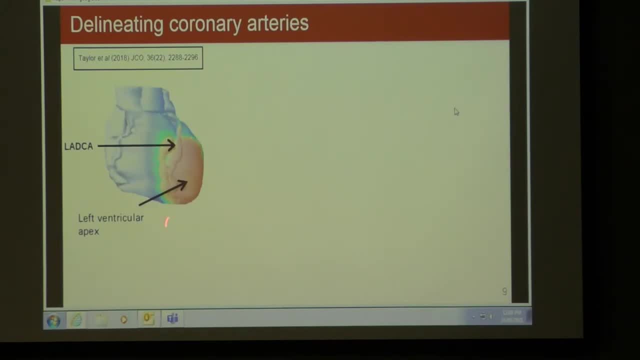 And I'll show you why in a moment. And that's something that we really want When we start to analyze the heart dose, Because we have lots of coronary arteries, Which are where disease can start, And we want to estimate the dose received by these different structures. 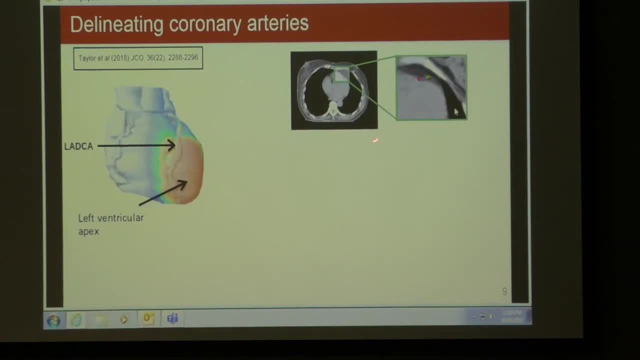 So why are they hard to delineate? So these are actually three maps: The manual contours of the left anterior descending coronary artery, The LADCA or LAD, And you can see there's no overlap at all, And atlas based methods rely on the overlap to define a consensus segmentation. 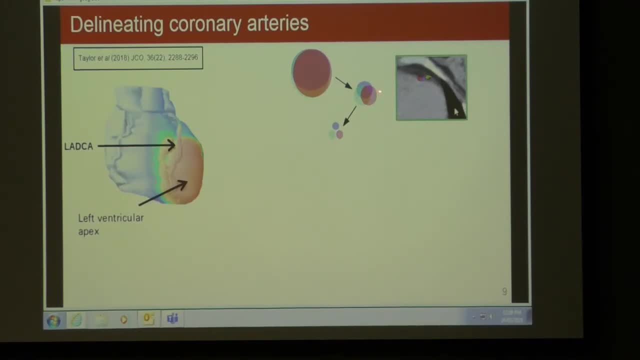 And even within a given precision. as structures get smaller, The amount of overlap reduces to nothing. So to overcome this limitation, We came up with a relatively simple algorithm That basically traverses the image And defines where the vessel should be based on these different estimates. 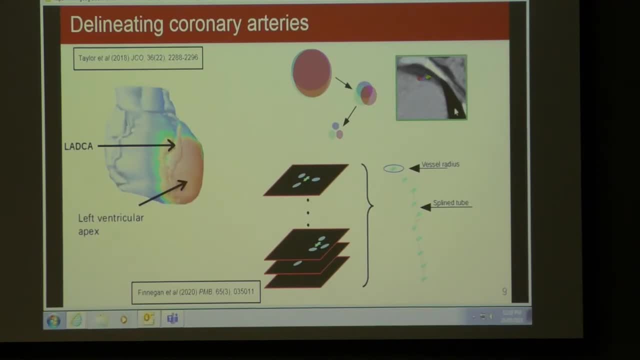 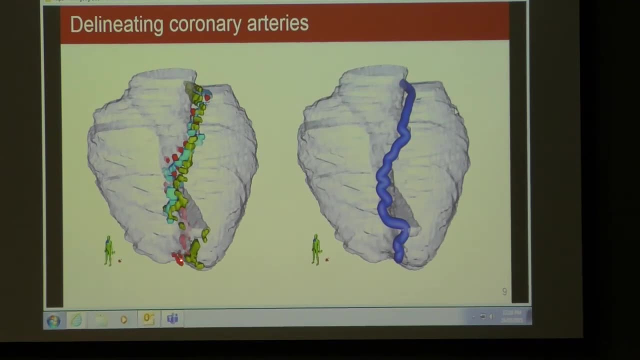 And then splines them together into a tube. So I think this picture does a good job at summarizing how this algorithm works. We have a lot of disparate estimations of where the LADCA is In the intraventricular groove here. 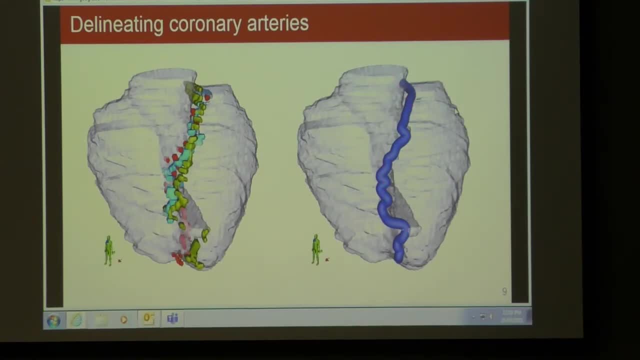 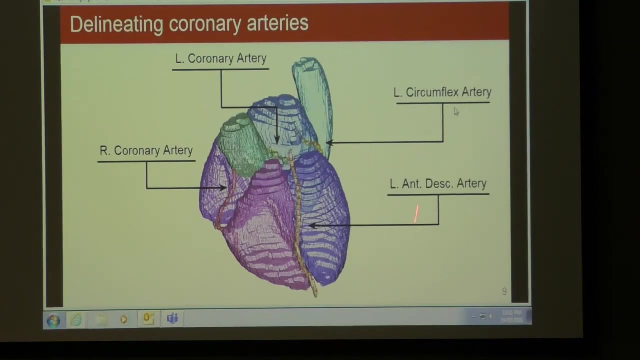 And we can combine these into a really accurate automatic segmentation Which we can define using a preset vessel diameter Which you can get from the literature Or potentially even adapt to individual patients. And we do this for all the different vessels, So we end up with an automatic segmentation of cardiac substructures. 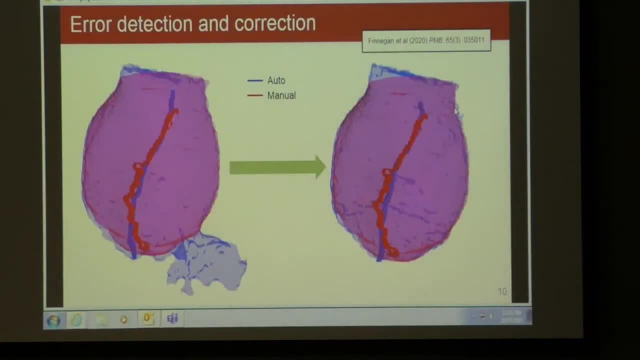 It looks a bit like this: Error detection. So any automatic segmentation is prone to errors, And we came up with quite a novel tool That can detect these errors automatically and remove them. So these are often the result of image misregistration When you're trying to map one patient image to another. 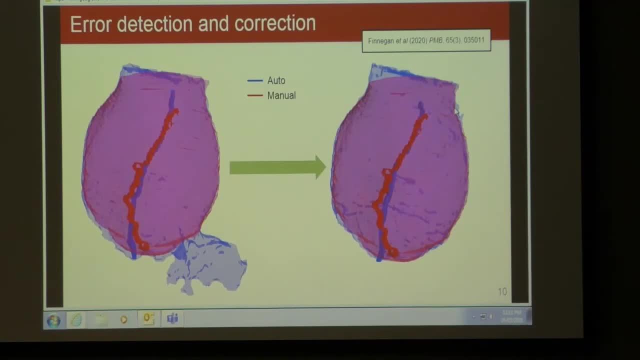 There's no way to do that with like a one-to-one mapping. Every patient's different, There's anatomical variation, There's image artifacts, And so you can quite often end up with errors, But thankfully, with this tool, we're able to reduce most of them. 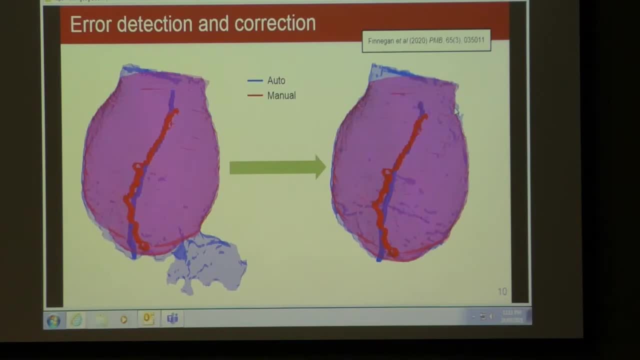 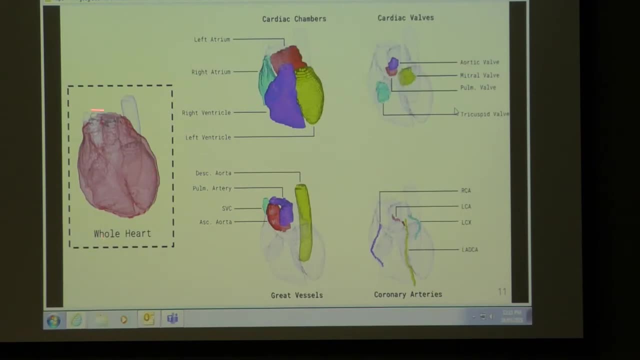 And, if you're interested, I can go through that in a bit more detail later, But for now I'll just move on. All right, So here's the story now, Instead of just looking at the whole heart, Which is what's done clinically- 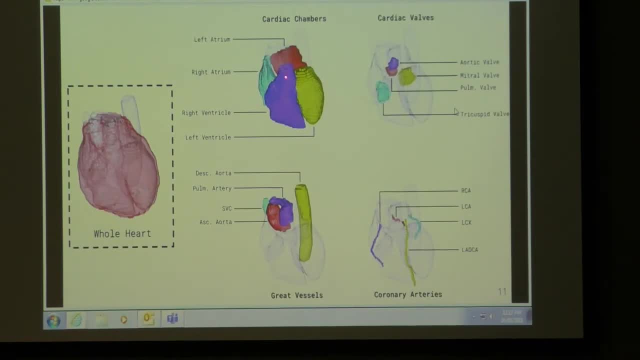 And also in retrospective studies, We can really start to break it down Into the individual substructures, Like the chambers and the valves, The vessels and the arteries. Which might be more in dose to these structures Might be more indicative of particular cardiac risks. 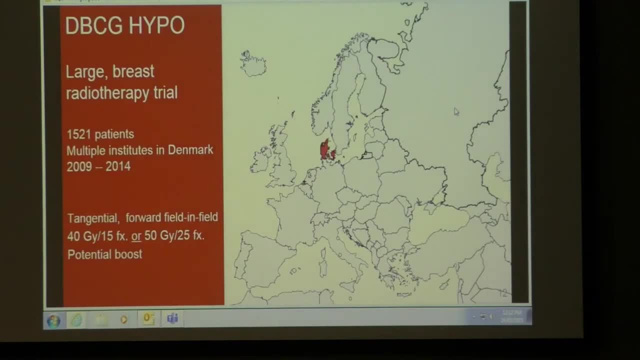 And something that we're obviously interested in. So one of the applications of this auto contouring tool Is to a large Danish radiotherapy trial data set. So a bit over 1500 patients, Multiple institutes across Denmark, And they're looking at the potential. 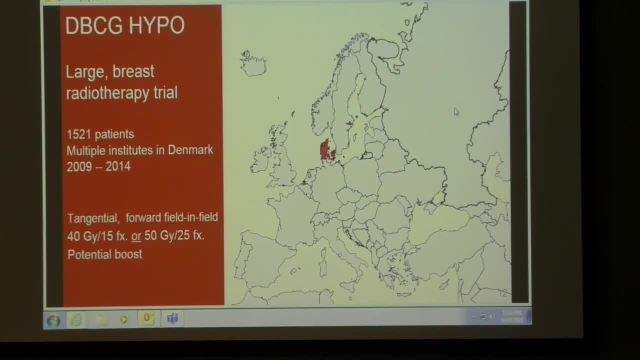 For hypofractionation, Hence the name DBCG hypo. The primary endpoint was actually breast induration, But obviously they're interested in Getting out as much information as they can, So they're looking at things like Other RT related morbidities. 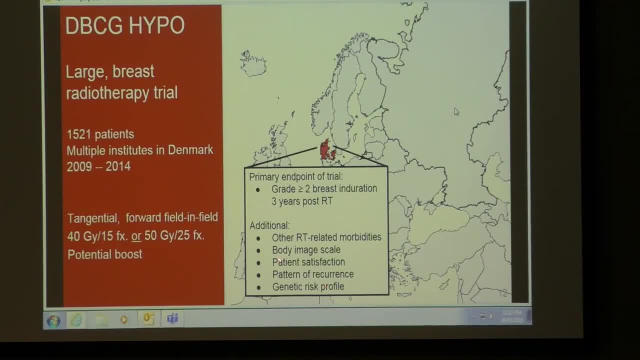 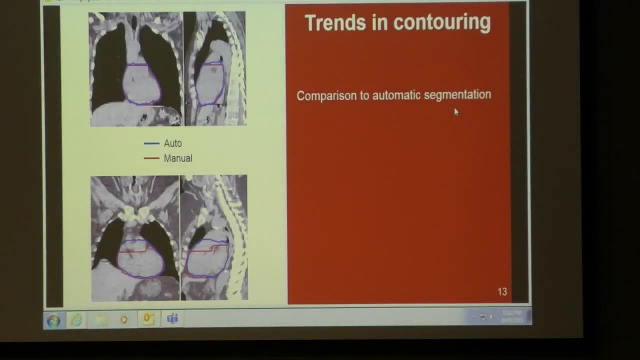 So that would be cardio toxicity, for example, And lung toxicity And patient satisfaction, Recurrence and so on. So using an auto contouring tool Can allow us to analyze How contouring practices have changed over time By comparing the manual contouring. 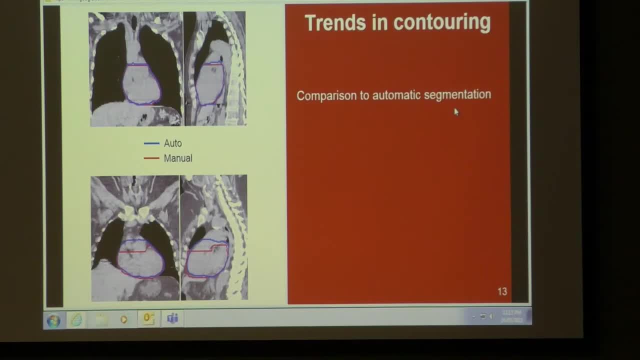 To these auto segmentations. So the automatic segmentation atlas Was developed using modern contouring guidelines And you can see the difference this has to manual contours In this bottom image here, Where this red contour here Is quite different from the automatic segmentation. 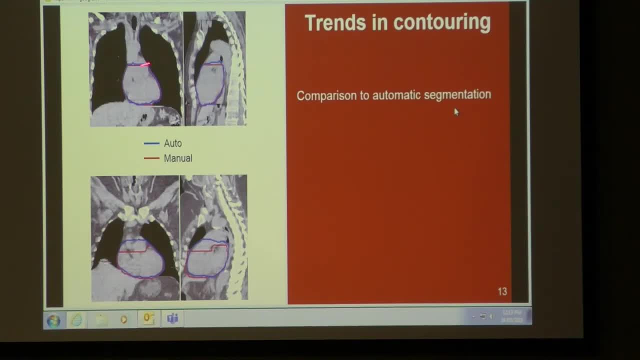 Which looks quite good. However, in some cases it's quite similar. So this kind of suggests That using manual contours In retrospective data sets Should be done with care, Because if we get dose information Just using the manual contours, We're obviously including the effects. 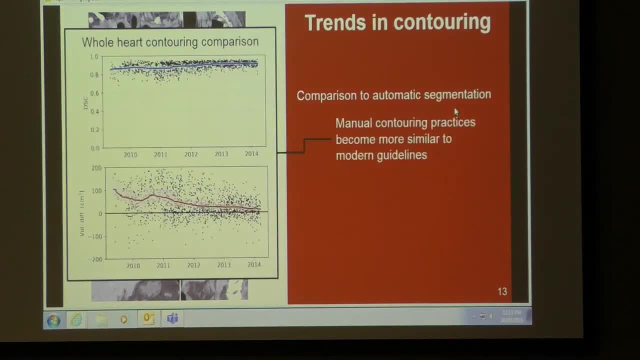 Due to changes in contouring, And this is looking at changes in metrics over time. So the die similarity coefficient Between manual and auto contours And you can see that it's getting better And also more consistent, Which suggests that manual contouring practices. 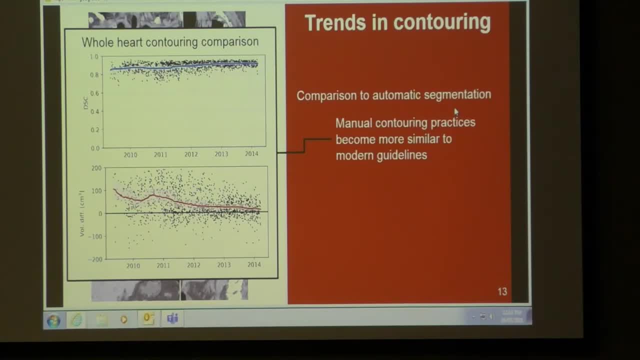 Are becoming more like The auto segmentation atlas That we actually use to perform the segmentation, Which is reassuring. I think this is important. This is looking at the volume difference Between manual and automatic segmentations And you can see that You know at the start of this trial. 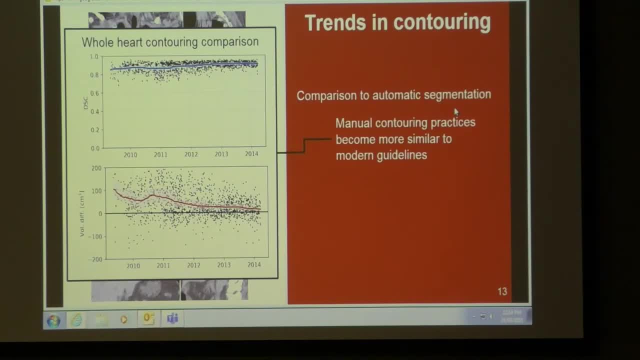 There's a very large systematic difference Between manual and automatic contours. Obviously this has a big impact In how we estimate dose parameters. But towards the end of the trial You can see that difference is minimized a lot. All right. Automatic contouring. 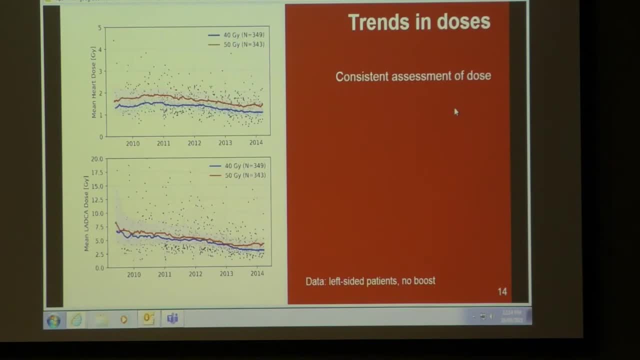 Translates to consistent dose estimates, Hopefully, And we can use that to analyze objectively How doses change over time. So Here is the mean whole heart dose And here is the LADCA dose. You can see that there is a general trend. 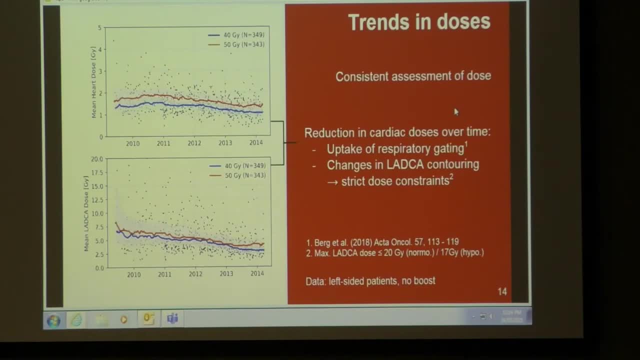 Towards decreasing doses, Which is great. Patients receive less dose To important cardiac structures. There's a couple reasons for this. There's a lot of deep inspiratory gating, Like deep inspiration breath hold, And there's also stricter dose constraints On, most prominently, the LADCA. 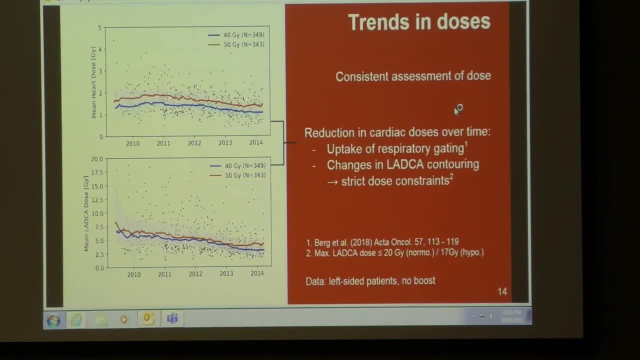 Which overall reduces The dose to the heart as well. But you can see that Still, patients are receiving quite a high dose To the LADCA And there are some outliers That can receive exceptionally high doses still, And this is using the auto contouring tool. 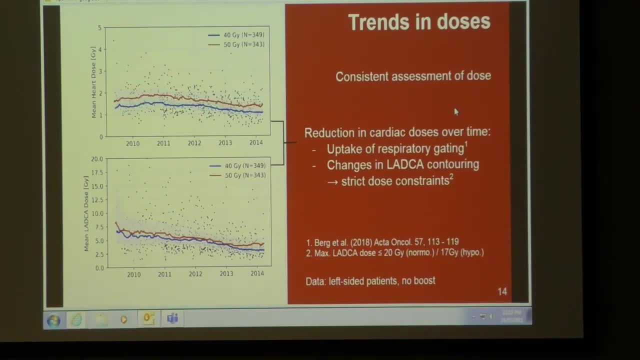 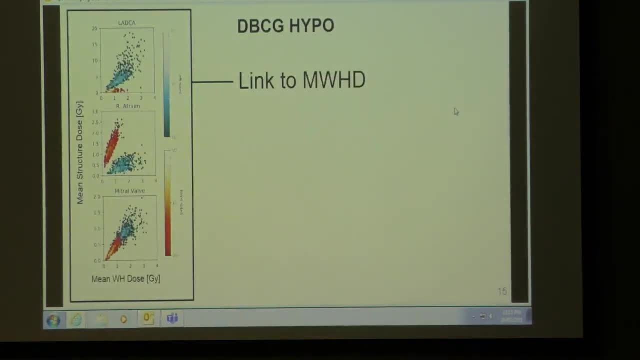 And not the contours That were actually used for planning, Which would likely Give a lower estimate Because of the constraints. Okay, Something that's interesting And something that we can use as evidence To support whether or not We should keep using mean whole heart dose. 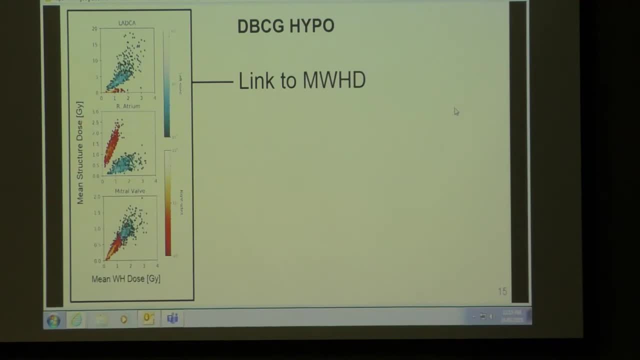 Is to look at the relationship Between the mean whole heart dose And the mean dose to different cardiac substructures To see how good a proxy it is For these different substructure doses. So sometimes it's a really good estimate You can see for the mitral valve. 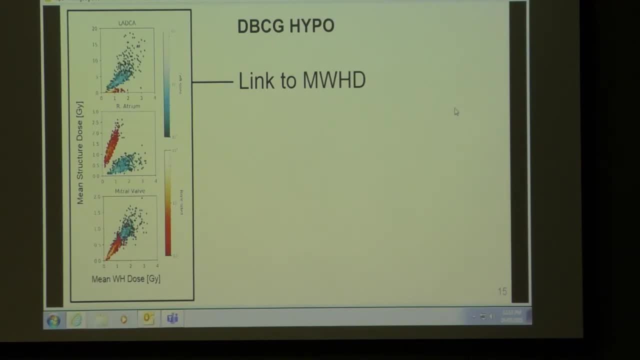 There's almost a one to one relationship Between the mean whole heart dose And the substructure dose, Both for right and left sided. So the text is a little blurry, But the hot colours are for right sided patients And the cooler colours are for left sided. 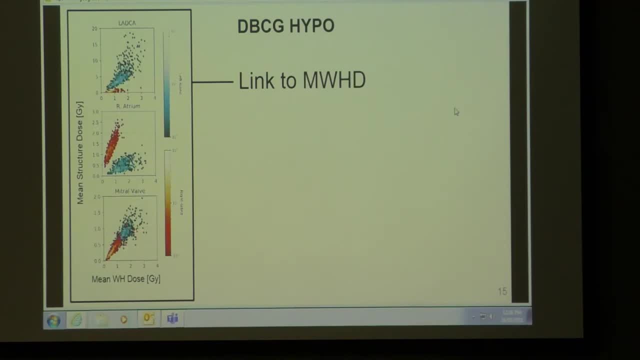 So it's unlikely that including Mitral valve mean dose Will provide any extra information. That mean whole heart dose doesn't. But that definitely isn't the case For some other structures Like the LADCA and the right atrium. 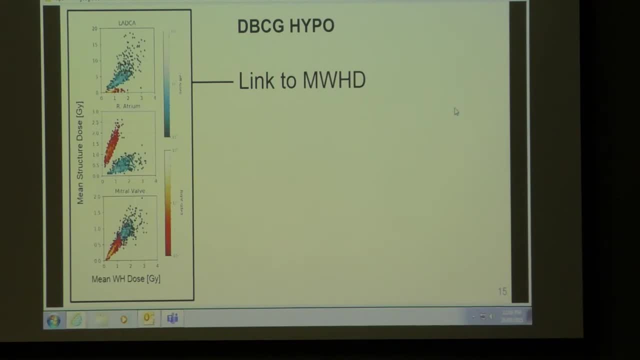 For which the mean whole heart dose Can be used, But can we include other Whole heart dose parameters Like V5, V10 and so on, And patient specific information Like heart volume To produce a model that can predict These substructure doses? 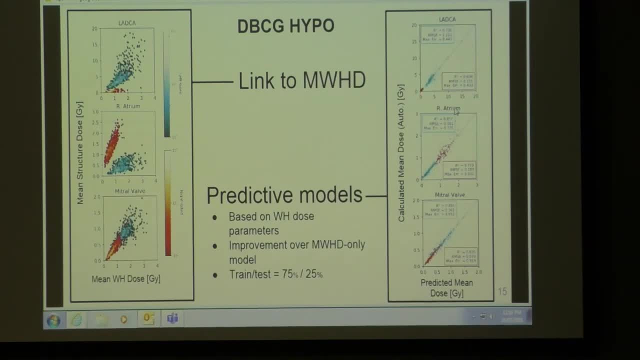 So that's what we did. Overall, we can do a pretty good job At predicting substructure doses, Using just the dose to the whole heart- Not mean dose, but a range of dose parameters And patient specific doses Like the size of the breast. 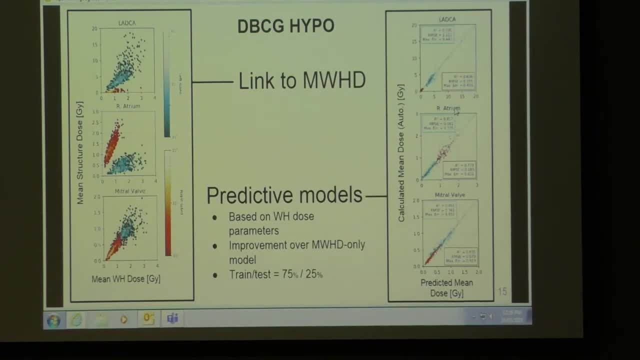 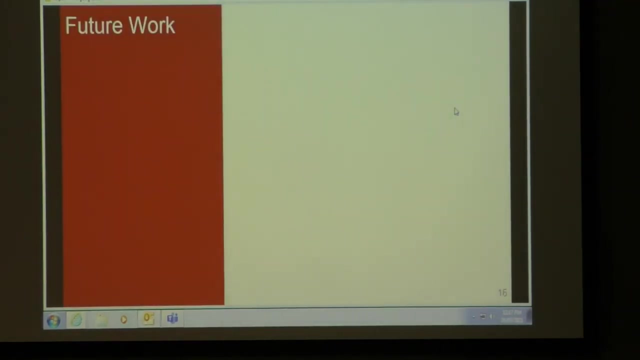 This is for breast cancer only, Where typically treatments Are a lot more consistent Than for lung cancer, for example, Where the tumour can move around in the lung. But interesting to note, Alright. So some future work With this cardioid auto contouring tool. 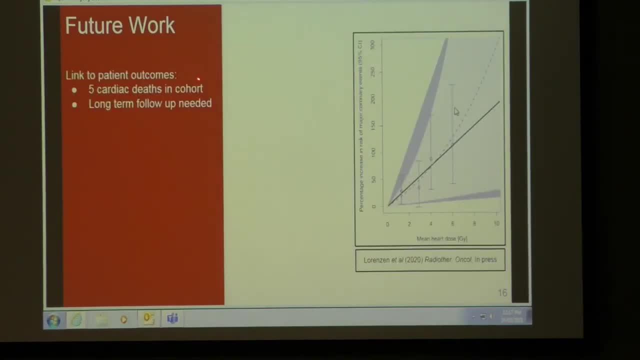 We don't have sufficient follow up To actually look at the relationship Between substructure, doses and outcomes. So far, there's only been A few cardiac tests. You'll note that the study ended in 2014.. So it's only about seven years. 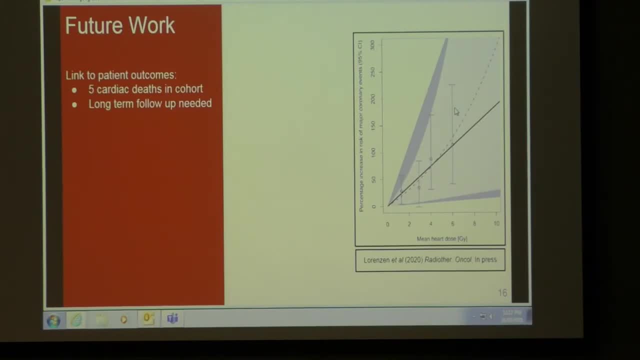 These toxicities can take quite a while To manifest as heart disease Or cardiac related mortality. So we'll probably have to wait Another 15 years for that, But research that has come out From our collaborators in Denmark Is suggesting that the increase in risks 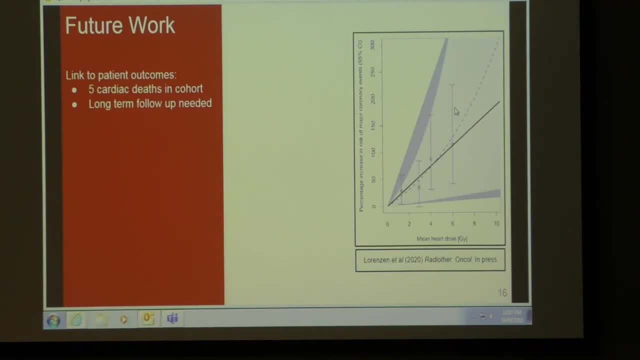 Is actually higher than previously thought, So it's something we should definitely Keep an eye on. I mentioned at the start A clinical implementation, And we've begun a pilot study At Liverpool Hospital Looking at how we can use this tool in the clinic. 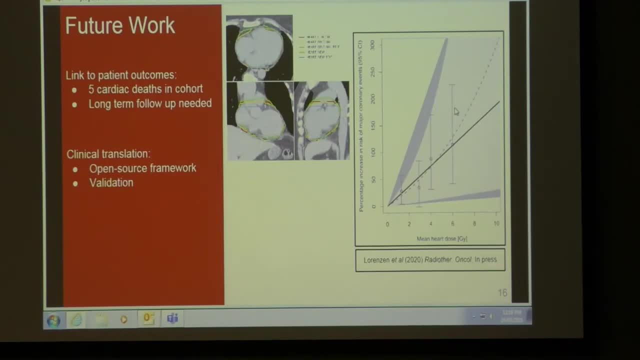 How it differs from existing auto contouring tools That might be available clinically, And something that I'm really interested in Is using automatic tools to better understand The uncertainties we have in estimating doses. So I'll just quickly talk about that now. 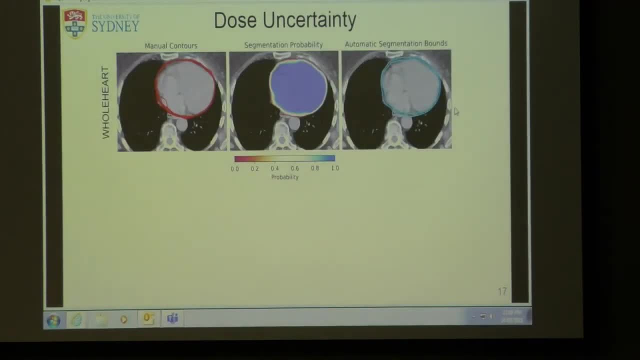 So, both clinically and in research, It's incredibly interesting To look at the uncertainty in dose, And one of the largest contributors To dose uncertainty Is from contouring, Or segmentation, Whether you use a manual method Or an automatic method. 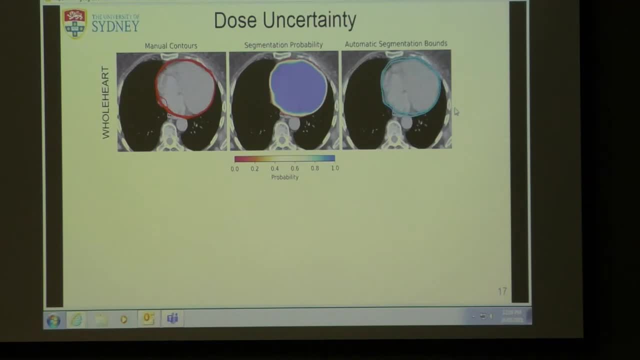 So we have a data set Where nine different manual observers Contoured the whole heart And we can use this variability in contouring To generate an automatic model That can estimate the segmentation uncertainty Of the heart contour. We can actually have a range of contours. 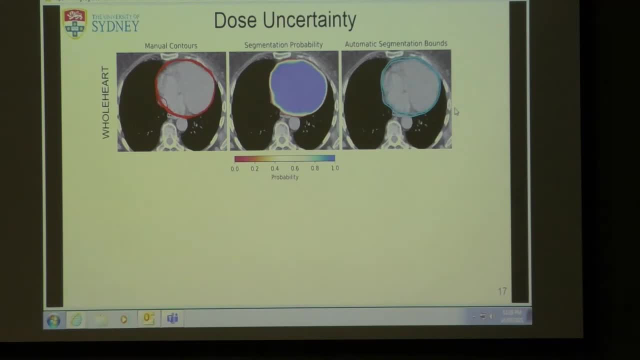 And this range of contours Encapsulates the uncertainty we have In the position of the heart Or the location of the heart, And that's derived from this probabilistic label map Which I was talking about at the start. That's generated automatically. 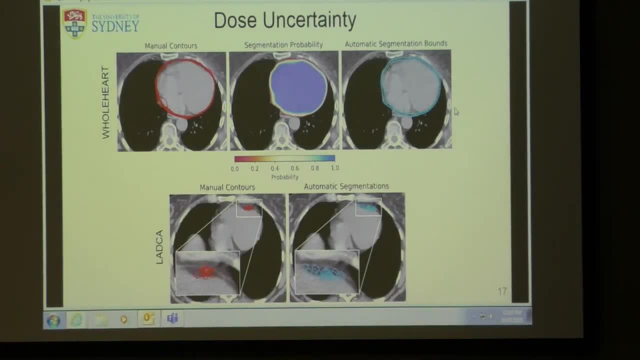 We can do something similar For things like vessels. It doesn't really make sense To make like a really big vessel And a really small vessel, Because it's not so much the size of the vessel But rather it's position, And so we can model variability in position. 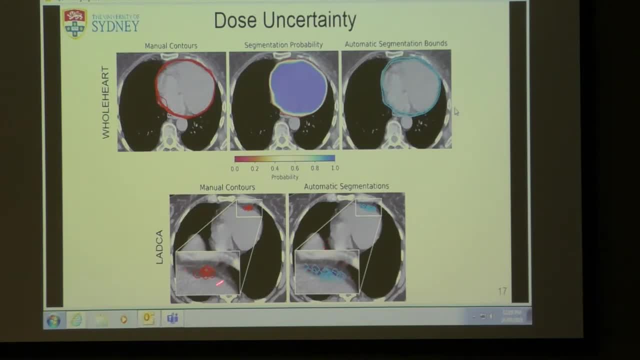 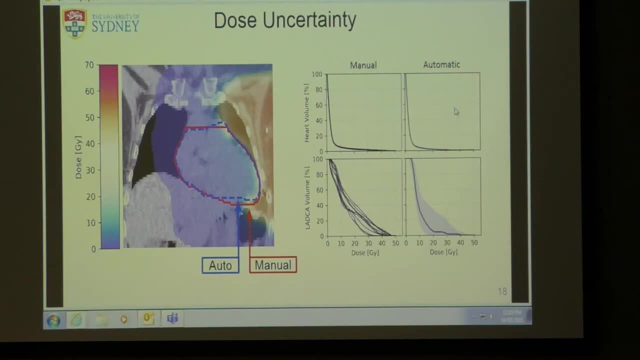 Using our automatic approach And compare that to manual contours, So what we end up with Is basically an extension To the dose volume histogram Or any dose parameters. That includes the uncertainty. So here's the DVHs For each of those nine manual observers. 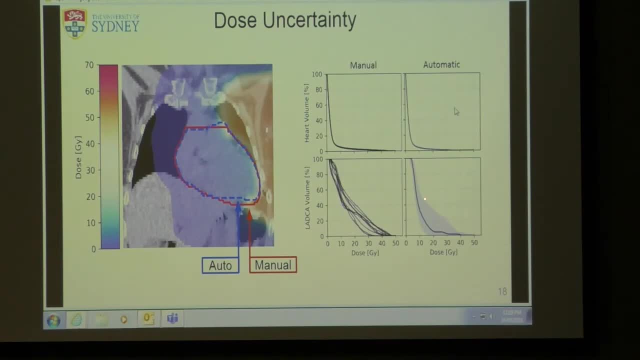 And here's our automatic estimate, With uncertainties derived Using that method I described. So interesting potential To be included, I don't know, Maybe in future research programs Or even in the clinic, You know if a clinician draws a contour. 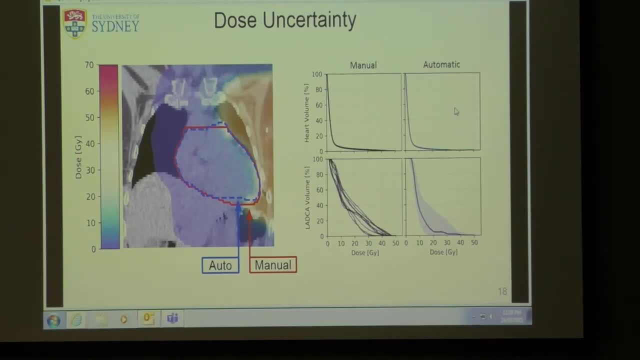 We could automatically generate a range in the DVH And that could be used To guide more robust treatment planning strategies, Because you know For an individual patient If the dose could be anywhere in this range. Maybe we want to try to make a plan. 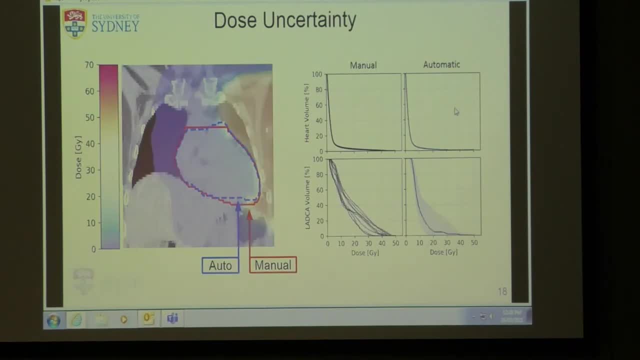 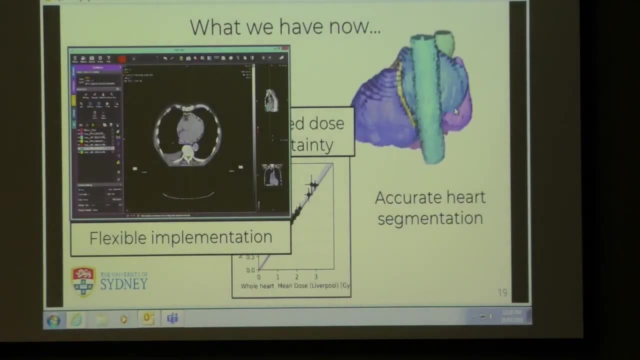 That results in a lower dose Than the normal contours. So what do we have? We have accurate heart segmentation, Model, dose uncertainty And a flexible implementation. We can use it offline In more of a research approach, Or we can use it clinically. 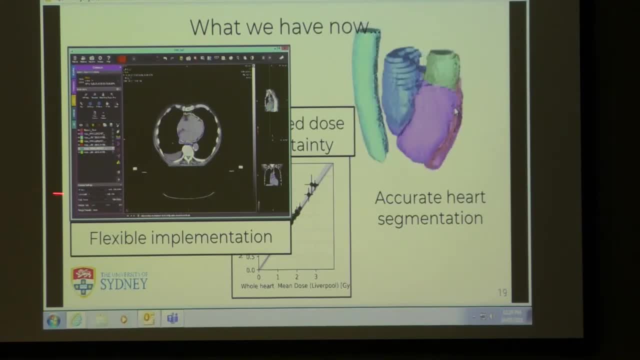 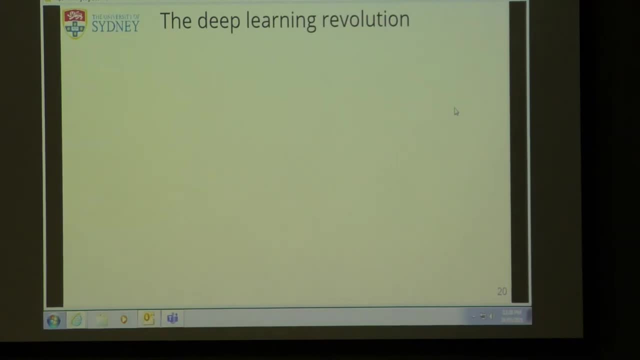 It runs on a server In our clinic And you can basically call on it from MIM. I'm not sure if people here have used MIM before, But it's a good tool. I thought I'd quickly mention deep learning Because obviously 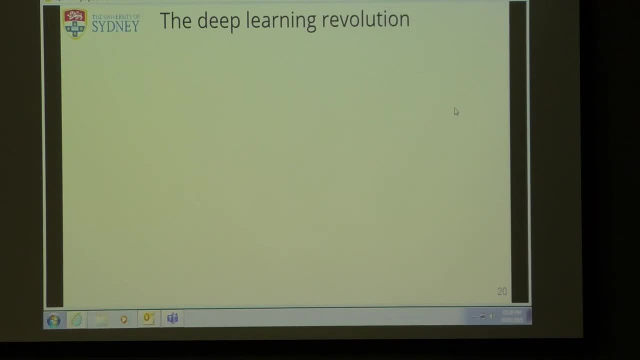 Deep learning is being used all over the world And being used in more and more different research projects, Especially things like auto contouring, And we've implemented An instance of the NN unit Which was recently published in Nature. And the NN unit. 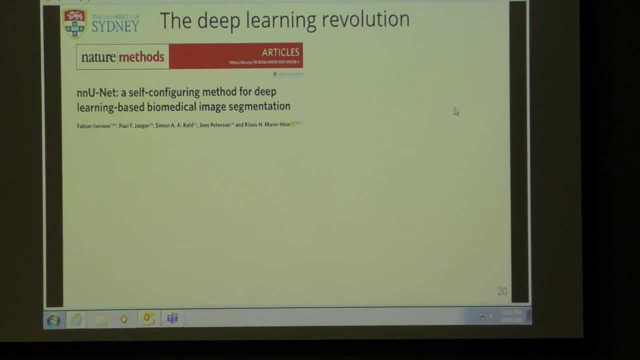 Tries to abstract The challenge of deep learning One step further By also trying to generate the optimal parameters For your deep learning model, So that you don't have to Spend too much time fine tuning How many layers and so on. 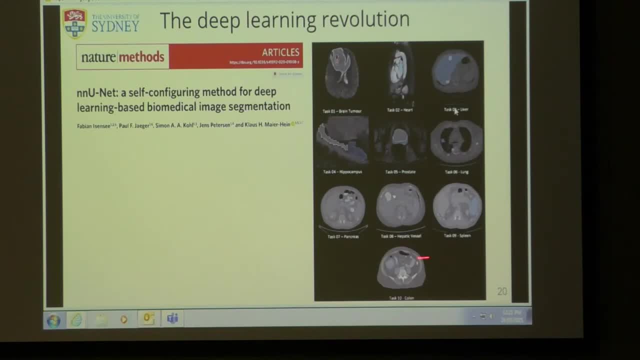 They did this by testing it Over a range of different tasks. You can see here There's some different imaging modalities- MR for the hard And CTs and so on- And they basically build up this library Of fingerprints. This image isn't displaying too well. 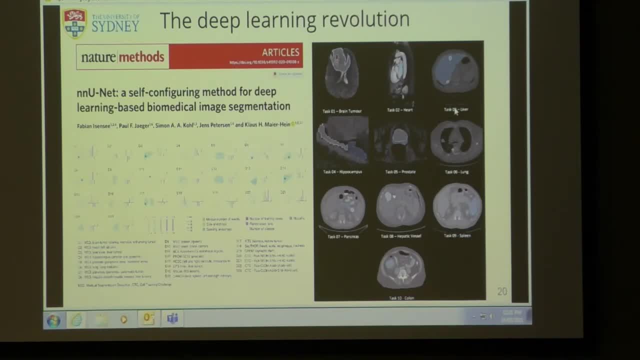 But fingerprints being a set of parameters That provides the optimal deep learning network For a given segmentation challenge. So how can we use this? We don't have sufficient data To include all the cardiac substructures. So far we only have 20 manual. 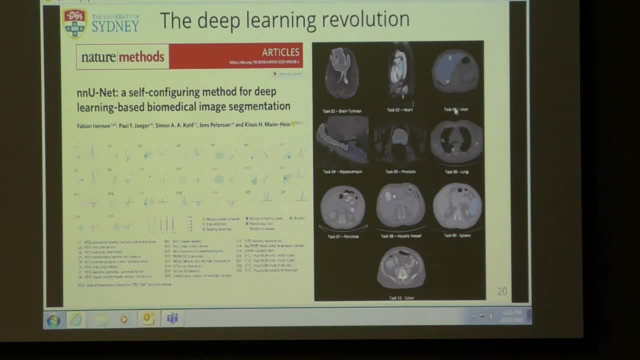 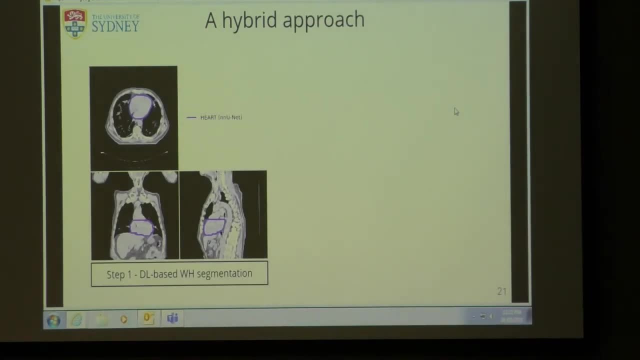 Manually contoured cases Which constitute our atlas, But what we do have Is a lot of whole heart contours. So we've developed a hybrid approach That first uses a deep learning network, The NN unit, To create a whole heart segmentation. 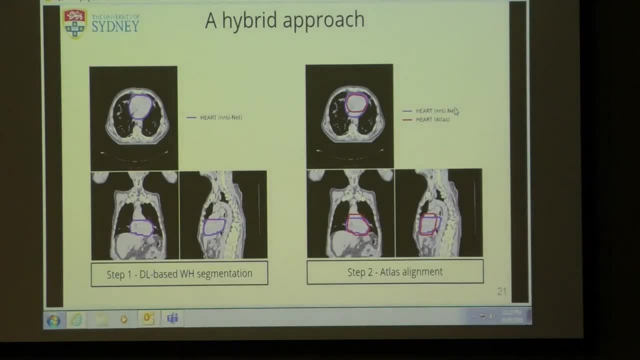 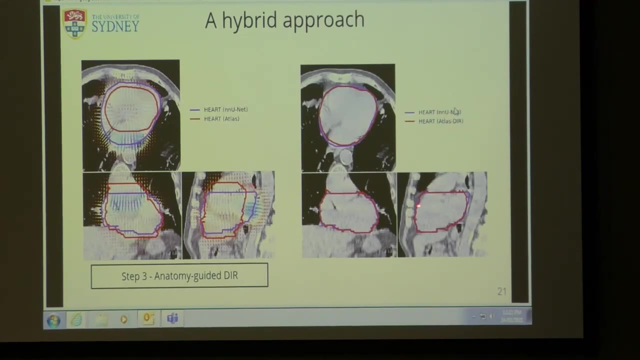 And then we map the atlases onto that. So hopefully These next few slides will make sense. So first we align an atlas Just using Deformable image registration. Then we use deformable image registration To basically At a voxel level. 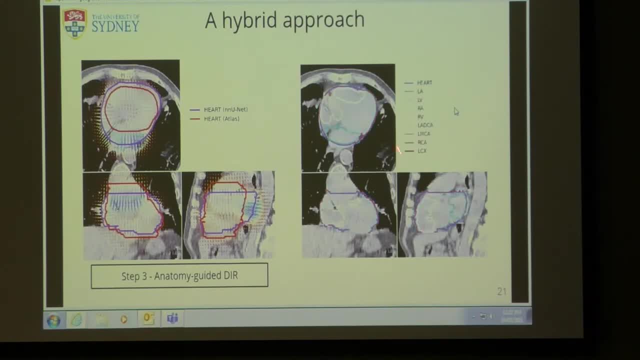 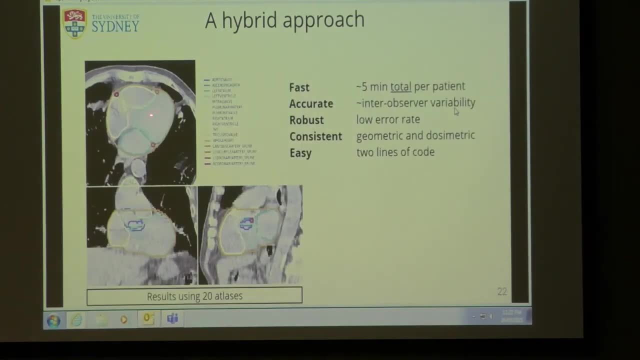 Map the atlas onto the individual patient. Since the atlas includes all the cardiac substructures, We can map those across too. Then we repeat that For all of the different atlases You can see here we get really good results, Especially for smaller structures. 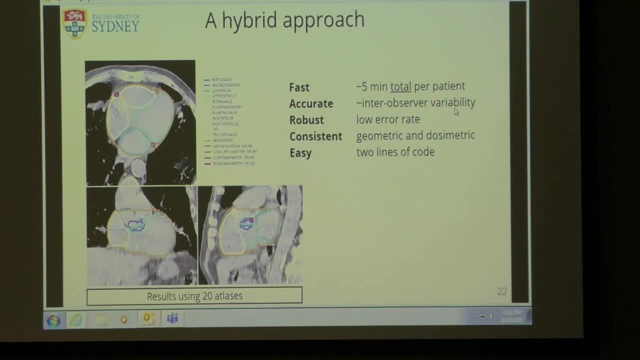 Such as valves, Which are notoriously difficult to segment, Either using an automatic method Or manually, Which has a lot of benefits to existing frameworks. It's super fast, Five minutes total. So from a blank image To every cardiac substructure contoured. 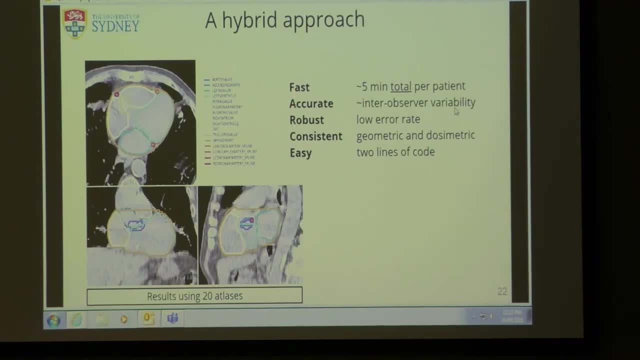 The accuracy is about At the level of inter-observer Contouring variability, So we can't really hope to do too much better than that Without moving to other imaging modalities Like MR That offer superior visualisation of substructures. 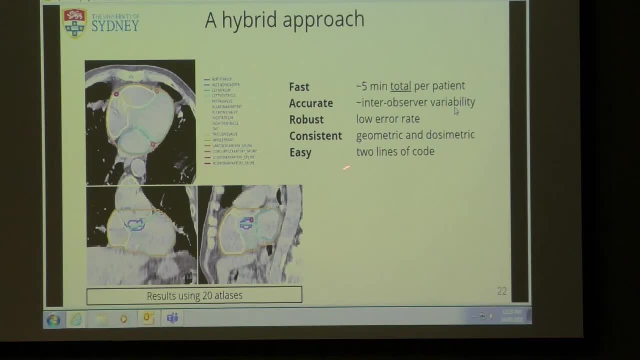 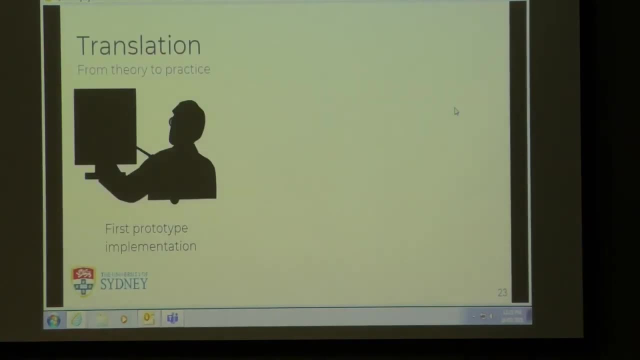 It's robust and consistent And it's super easy To generate these segmentations, With obviously a lot happening Under the hood. Alright, This didn't display, That's okay. So there's lots of good reasons Why this cardiac segmentation tool was developed. 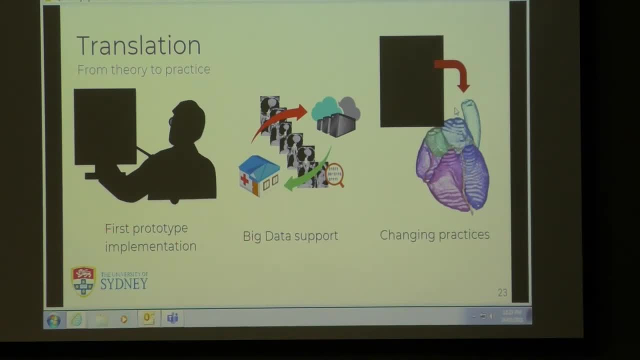 For clinical implementation, To support the research, Using big data sets, Retrospective data sets That contain a wealth of information we can use To develop better risk models And to change practices. And RTS To delineate cardiac substructures. 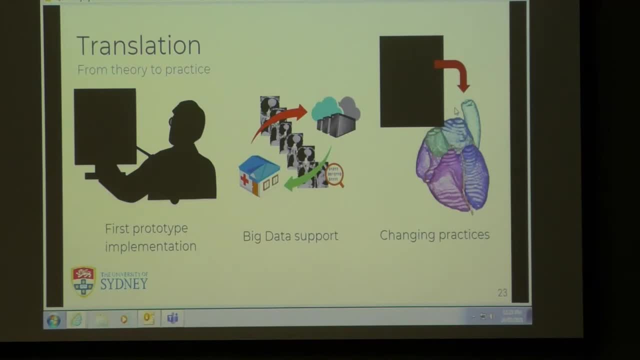 For every patient, Extremely time consuming. But if they can do a whole heart contour, Then we can just map across the cardiac substructures And you know Whether or not this becomes something in the future That's used, We'll see. 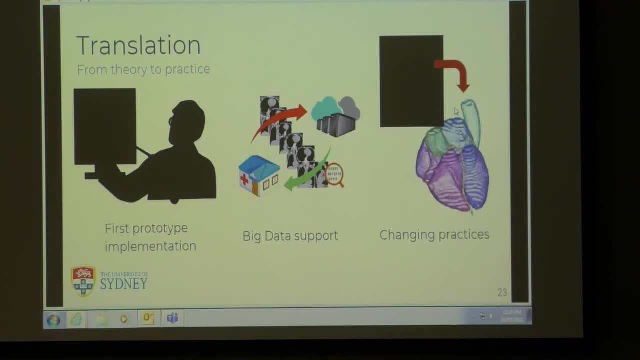 Alright, So that's the cardiac project. I don't know if anyone wants to ask questions now Or if we want to move on to the prostate arts project. I have two comments. One is fixable. So looking at death rate For the Danish study, 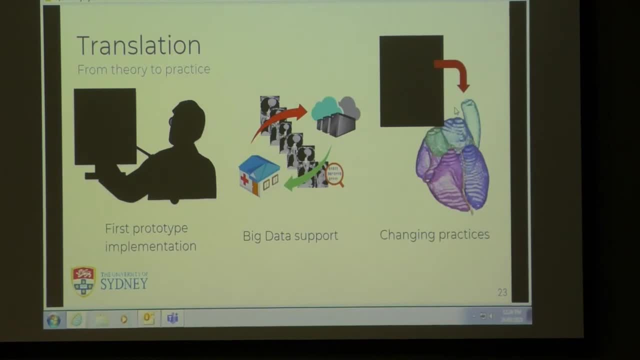 Is probably the wrong thing, Because they get chest pain And have a stent And they never die from their heart disease. The second comment is: I really think that the thing that's going to change practice Is your substructure segmentation. 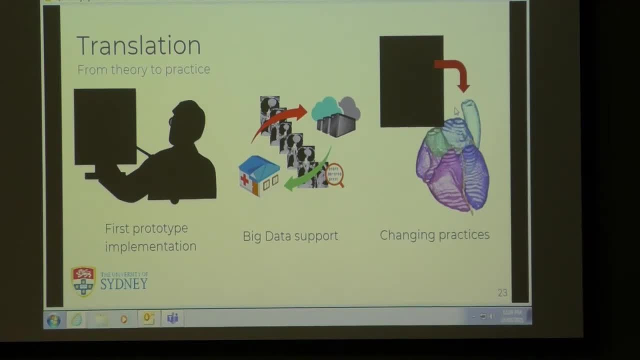 Mainly because radiation oncologists Haven't been taught Where the LED is Or where the valves are And we are actually artificially, When only certain structures Are really important. For sure, the valve would have some damage If you pass radiation through it. 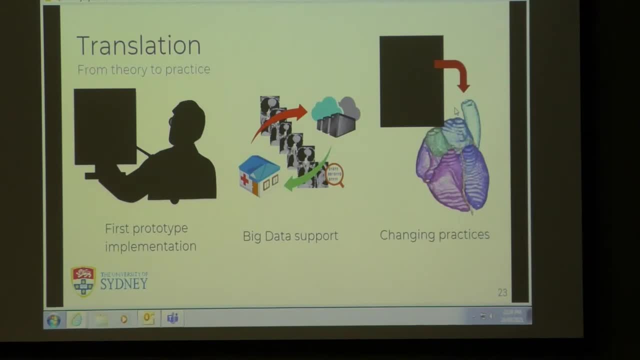 Or the cardiac disease. These are the things that we need to Actually measure for future studies, So that we can know what the tolerance, Because it's not the tolerance of the muscle That's the problem, And the other structure That you haven't outlined. 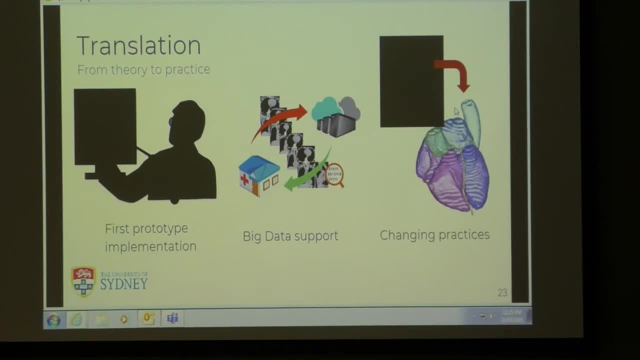 Is the pancardium, So that the pancardium can Possibly affect Substructure segmentation. So I think you're on the right track With substructure segmentation, Which essentially Number one, We don't even know where these structures are. 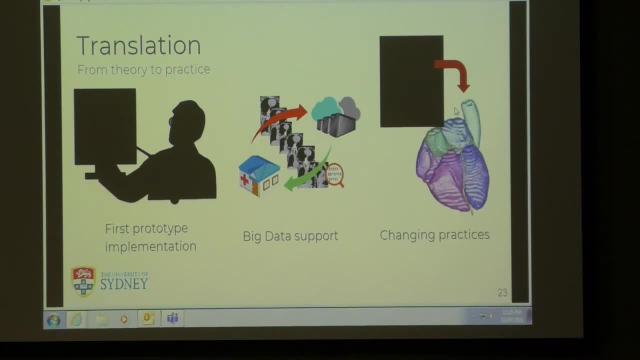 We've never practiced them. And number two, It's very time consuming And every valve That would really change practice. Yeah, Fingers crossed. The big data sets that you've used: Are they Setting up? something like this Is always the time to find. 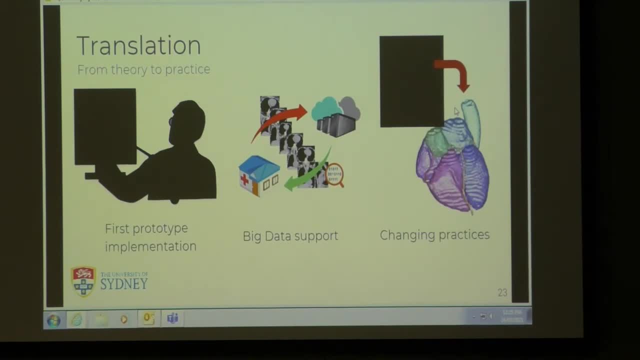 To get the libraries To get the data. Yeah, How would you, For an institution, Get that data set Available Free, Or where can you get it? Yeah, It's great And, as Suki says, It's. 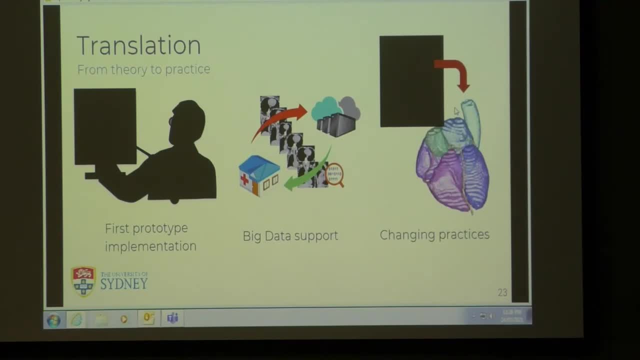 Setting up any of these projects. Well, This is a project, But setting it up in the clinical setting Is really difficult. Yeah, It is For sure. How do we get to get these big data sets That we could possibly even start? 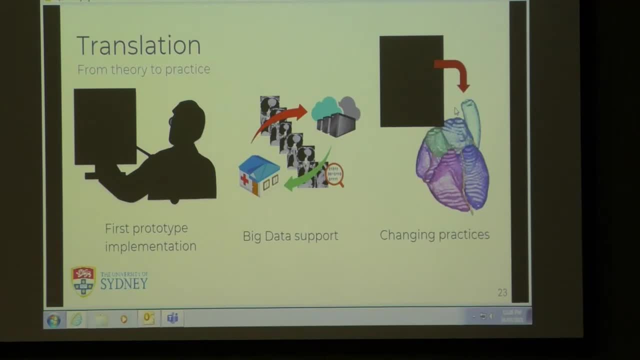 Yeah, So It's a good question And, you're right, It's less relevant. Yeah, So We're part of the OSCAP network At Liverpool Hospital, Which is an international collaboration That aims to develop a distributed system. 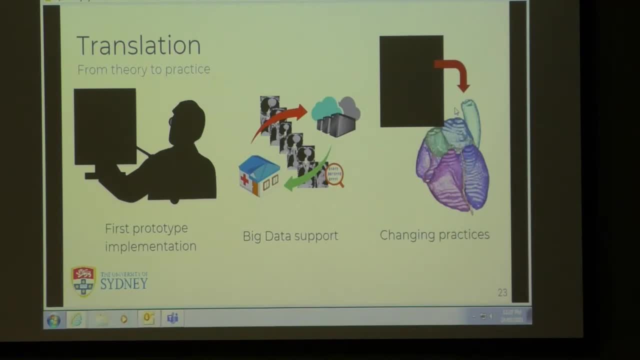 To basically train machine learning models. So Use data from multiple different institutions And use similar models, So for example, An automatic segmentation algorithm At each local institution, And then aggregate the data With ethics requirements And so on. But what we're doing? 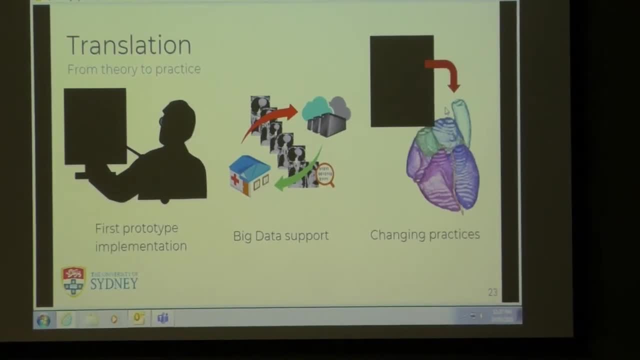 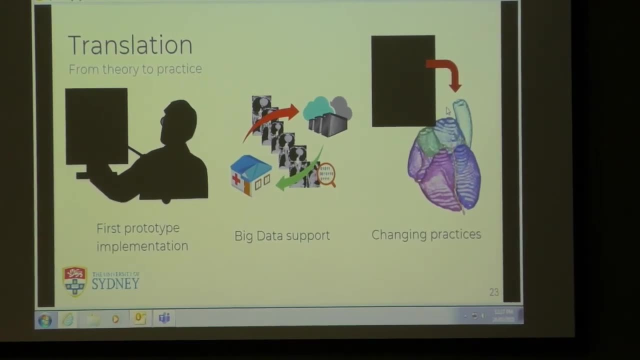 Is installing software At each computer That we can modify and update And access local registries. So I hope that answers your question a bit And I agree completely In terms of implementing in the clinic. It takes a lot of validation. 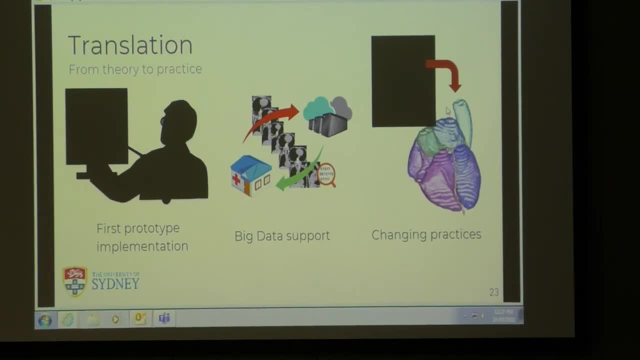 For a tool to be used And for something like cardiac substructures, For which we don't have dose constraints. There's not necessarily We don't get them, Because what do we do with the information? That's right, Yeah, Yeah. 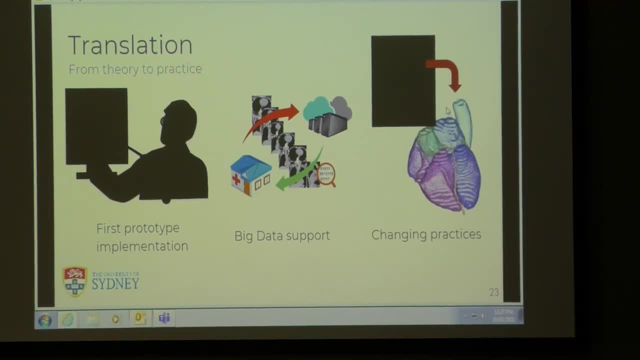 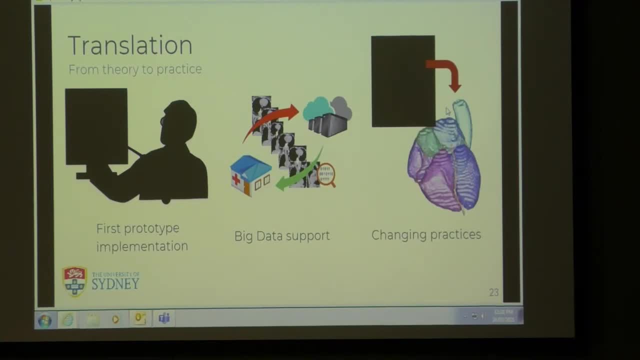 I suppose it's the best we can do With what we have currently, And that's why something like this tool For estimating uncertainties in dose I think it's really important. You know, I talked about from the point of view Of contouring uncertainty. 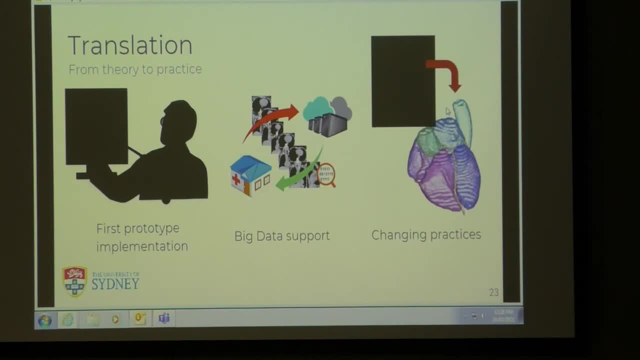 It's a lot of uncertainty due to motion. There's set-up uncertainties, There's a whole lot, Which is why we tried with DLBH. Yeah, Some of them. Yeah, Obviously the half. Yeah, Don't stop that, Stop that. 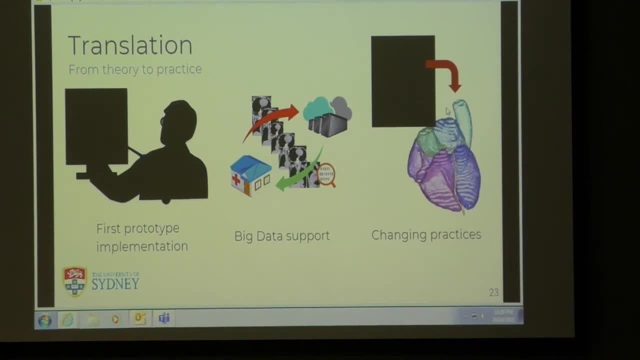 I just had a question about the contouring itself. It appears that each of your sub-contours are separate structures, And how does your algorithm deal with overlapping structures? Yeah, Yeah, it looks for overlaps in structures that shouldn't overlap Like the chambers. 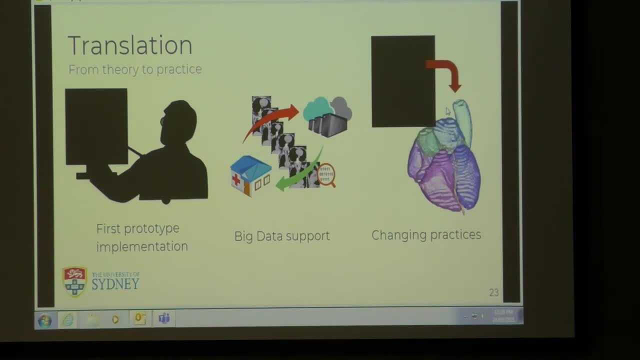 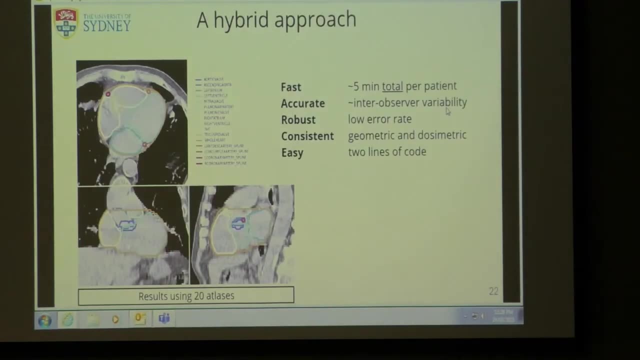 You know, one voxel should only be one or the other And yeah, it just assigns it to the largest one normally. But for some structures, you know, like the valves they do overlap, They do bridge the gap between different chambers. 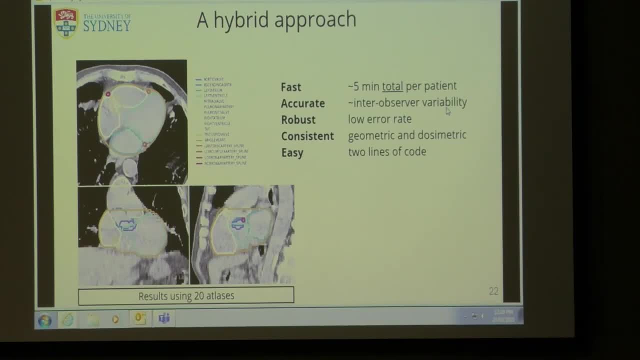 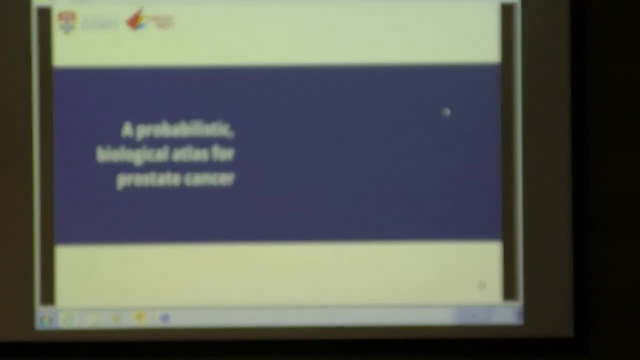 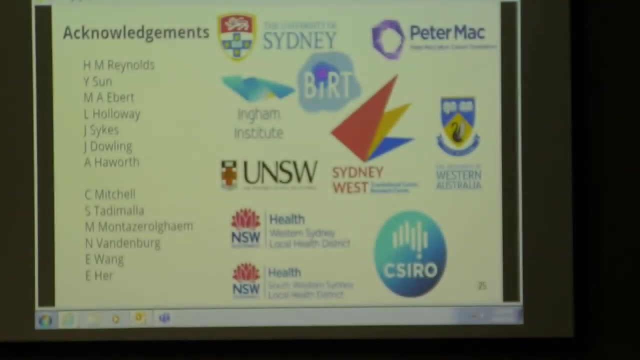 The colours aren't really showing too well here, but valves do move across here. Yeah, All right, Let's move on to a probabilistic biological atlas for prostate cancer- So something completely different- And also want to take the time to thank everybody who's involved in this project and has contributed. 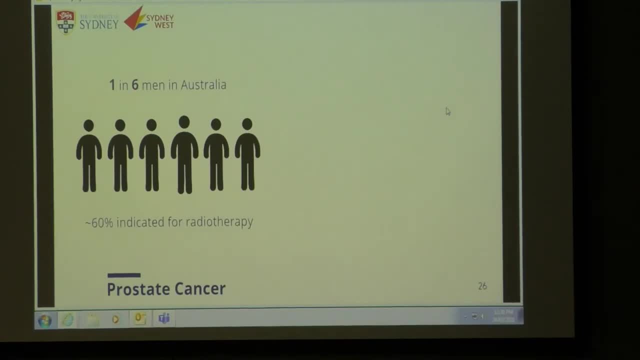 Okay, So prostate cancer is one of the most common cancers in men And a lot of patients benefit from radiation therapy And the current standard, The current standard of care, is to deliver a uniform, consistent and homogeneous dose to the entire prostate volume. 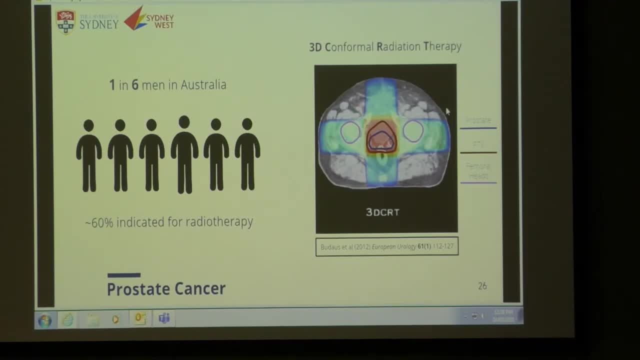 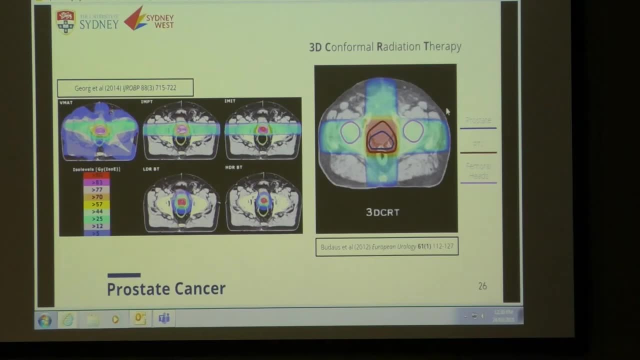 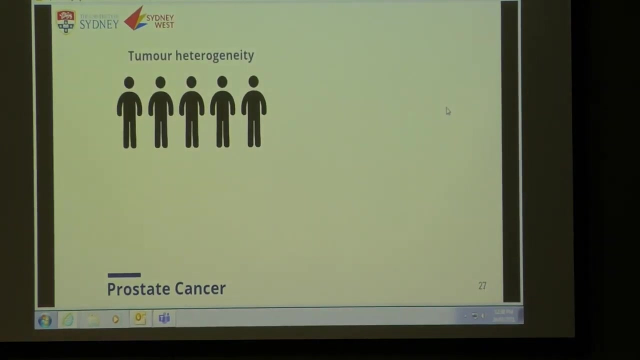 This image here is for 3D CRT, which is used quite often. But even for more advanced treatment modalities it's the same story: trying to deliver a uniform dose to the entire prostate volume. But this ignores the fact that everybody is well aware of that tumour. heterogeneity is present. 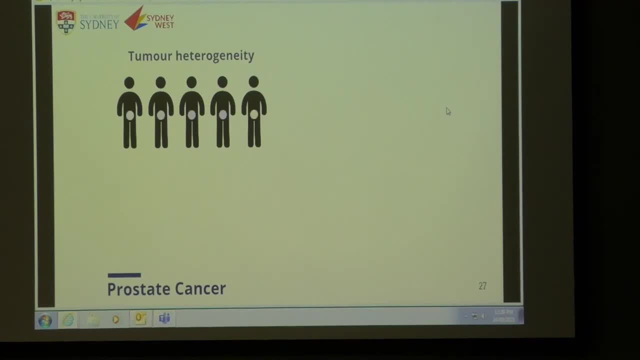 You know every cancer is as individual as the people diagnosed. You know every cancer is as individual as the people diagnosed. You know every cancer is as individual as the people diagnosed. But further than that, even within a single tumour, variation in biological characteristics of the cancer cells across the tumour affect how it responds to radiation. 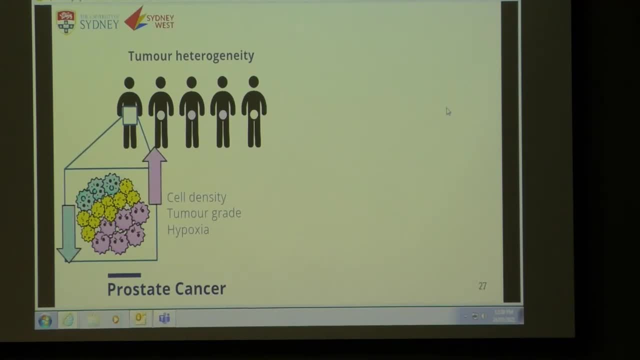 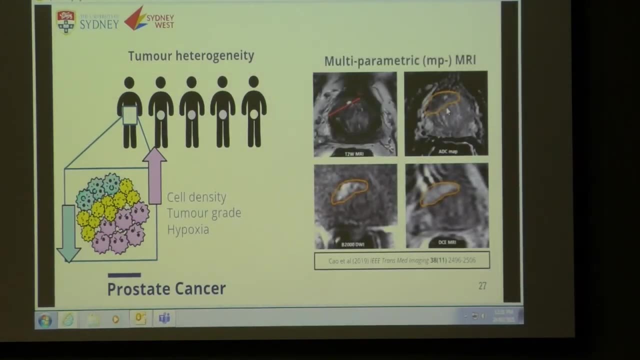 And suggests that different parts of the tumour require more or less dose to achieve adequate control. For prostate cancer, multi-parametric MRI is becoming more common in routine management. It's a sequence of different MRI scans. It provides a lot of information. 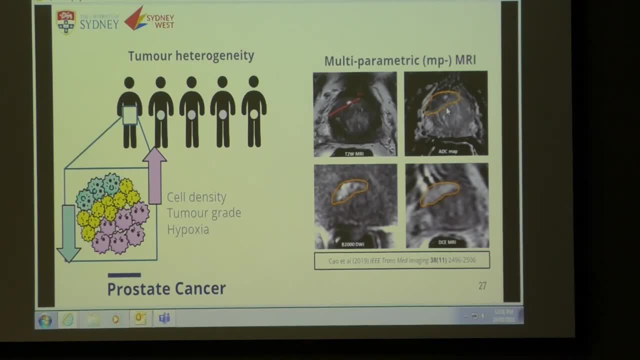 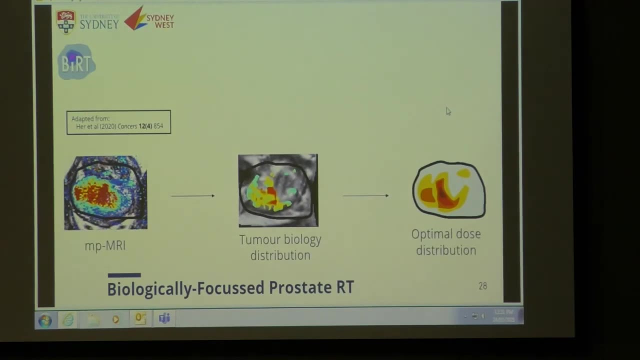 It provides a wealth of information about the underlying tissue characteristics, like diffusion properties, information on the blood flow and perfusion, And this can be used to generate quantitative maps of these underlying tumour characteristics. Which brings me to the aim of our research group, which is to use multi-parametric MRI to derive three-dimensional maps of the tumour biology. 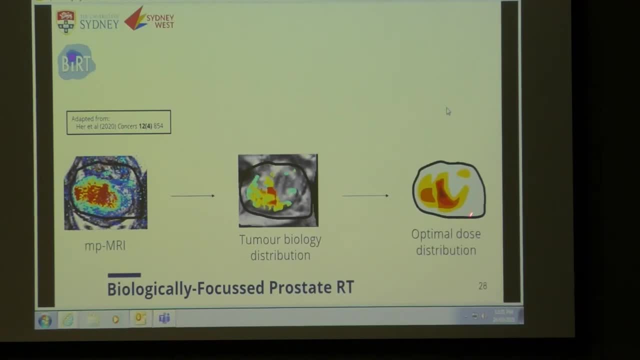 Use this information to derive a biologically optimised dose distribution That delivers more dose to where it is needed and less dose to where it isn't. The current AI models that we've developed to achieve this are limited in their accuracy, And one potential method to improve the sensitivity and specificity is through the use of atlases. 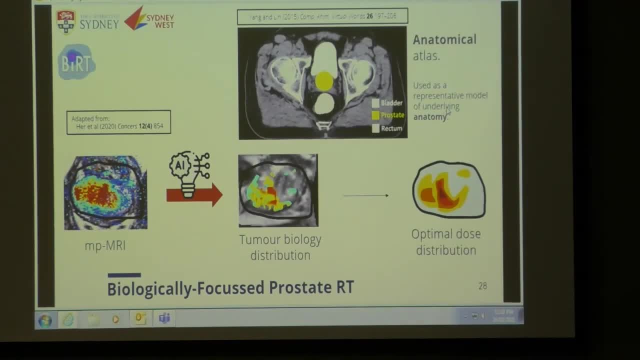 Atlases are common in radiation therapy already And they serve as a model of the underlying anatomy for patients. There's been a lot of evidence to suggest that atlases can improve the sensitivity and specificity of the tumour. There's been a lot of evidence to suggest that atlases can improve the sensitivity and specificity of the tumour. 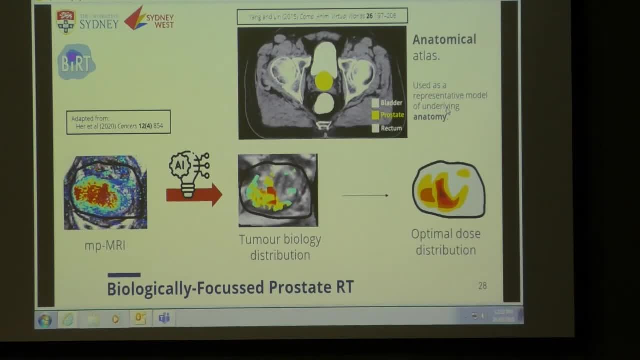 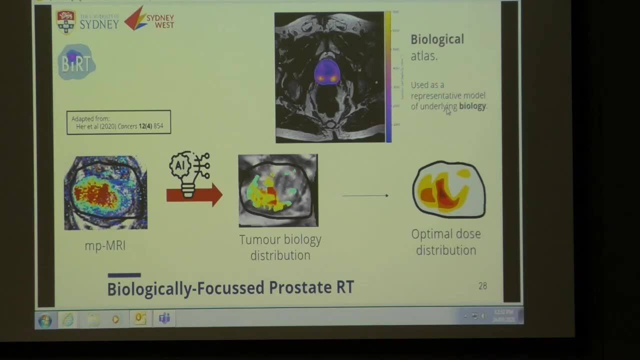 But what are thes? if it's developed? Atlases can improve the consistency and accuracy of defining anatomy. So why not go one step further and define a biological atlas and use that to improve the consistency of defining biological characteristics? That's our thinking. 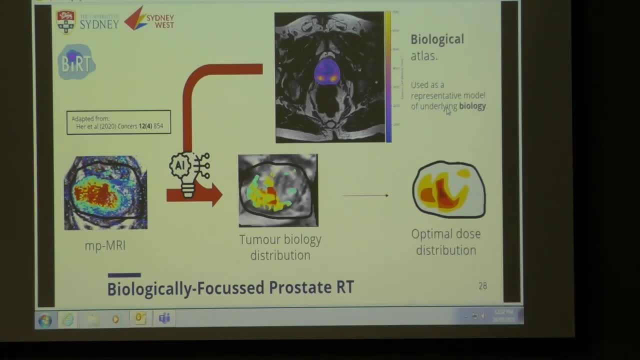 So we aim to use these in conjunction with existing AI models to reach the sensitivity and specificity necessary to be confident in our predictions of optimal dose distributions. As well as that, they're also really interesting to see on a population level where tumours occur, characteristics of them. So this is a quick summary of the AI predictive. 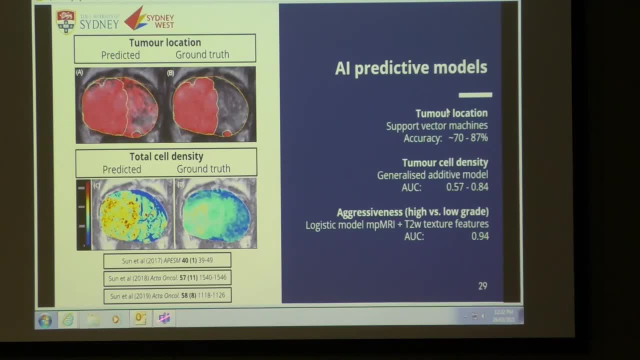 models we've got at the moment. A lot of this work was done by Yu Sun, who's a researcher in Melbourne now, but previously at Sydney, who developed a range of different machine learning tools to estimate tumour location, tumour cell density and aggressiveness and achieved overall pretty good results. but 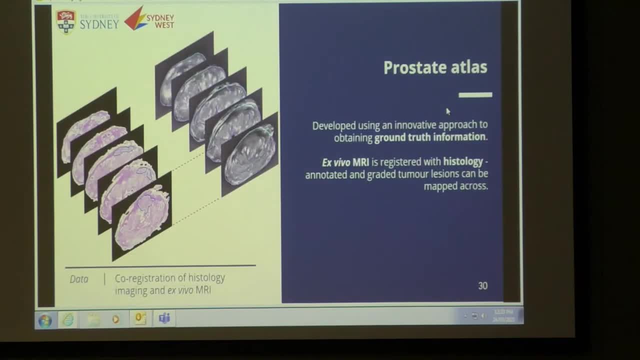 as I've explained, we want to take this to the next level, So I'll describe how we construct the prostate atlas and show some preliminary results. So one of the main points that sets this work apart is the innovative approach we've taken to obtaining ground truth information. We want to map the information about where. 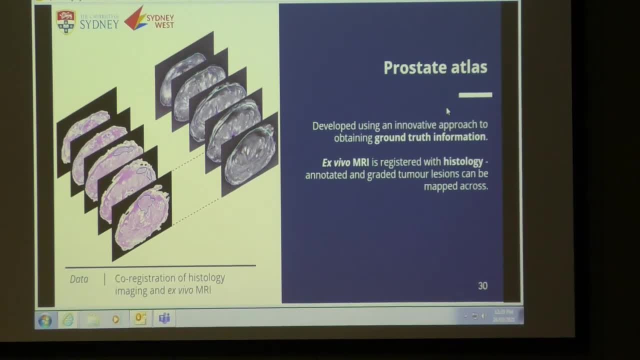 tumours are, and their grade and cell density and so on, to the actual MRI images, so we can use that to derive models. To do this we use a specially custom-made sectioning box into which a prostate is placed after it's resected. then it's imaged in the MRI machine and then we take slices. 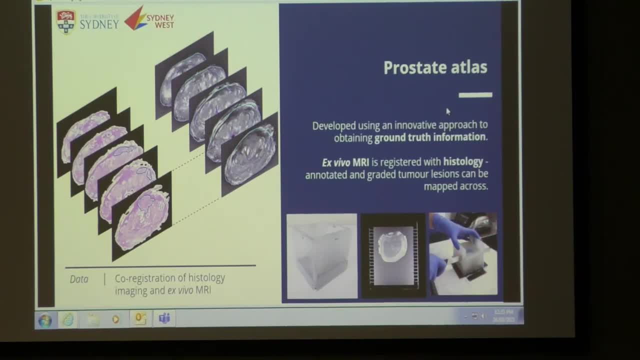 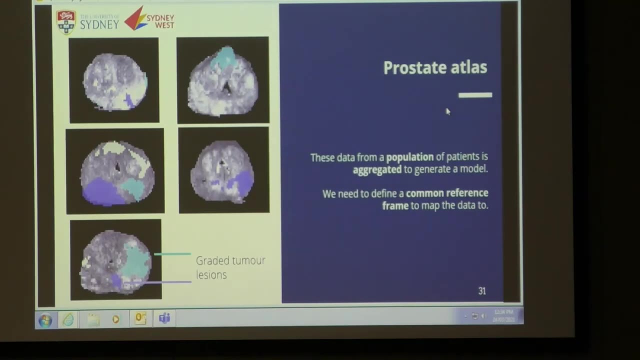 and analyse those slices using histopathological analysis, and this allows us to map information from the histology directly onto the MRI with minimal uncertainties. Once we have this information for each patient in the cohort, we want to aggregate them into a common reference frame so that we can generate this population level data. So 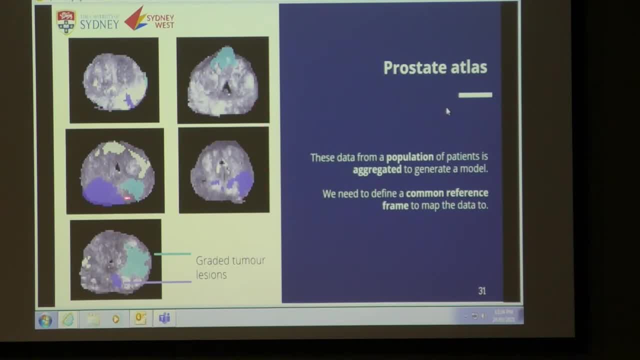 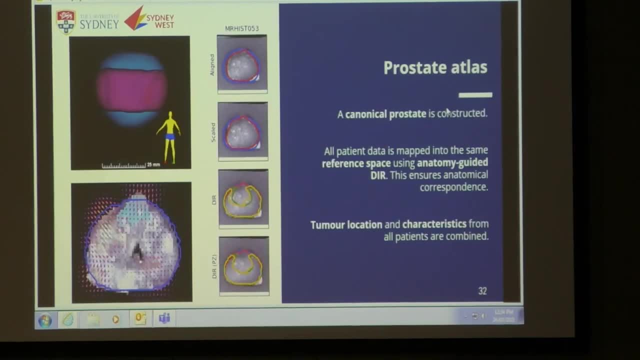 there's a lot of variability in the shape, the size, the extent, the orientation. everything you can imagine of these different prostate scans and the tool that we use to align them is deformable image registration, the same tool we used for the cardiac project, interestingly enough. So here's a. 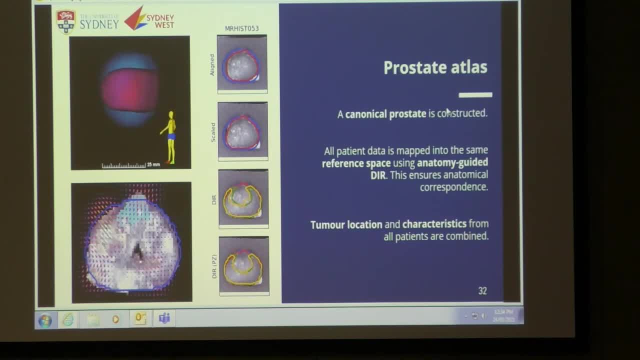 rotating model of our canonical atlas. This serves as like a reference to which all the other data is co-registered, And you can see here's an example. there's some vectors here showing how we deform this prostate to match it to the reference, so that we can align each. 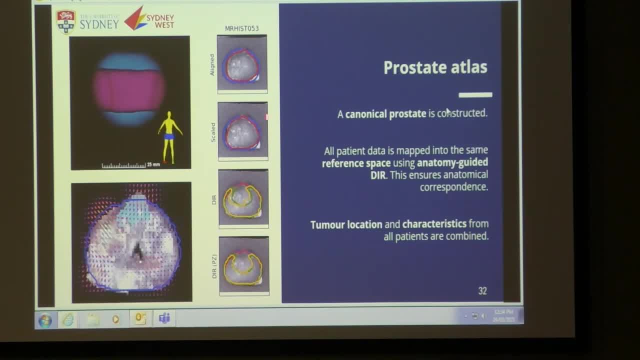 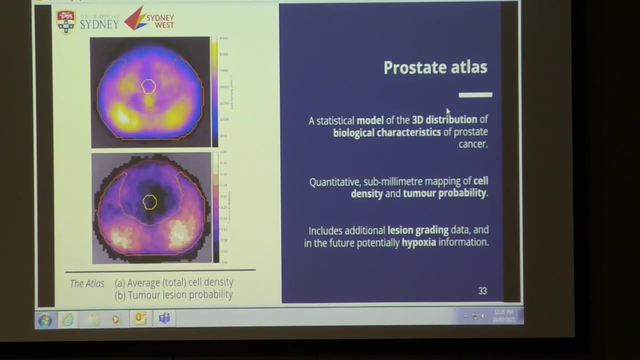 voxel. It's actually a four stage process. so we do alignment of the prostate, we scale it, we use deformable image registration to match the whole gland and then another stage to match the peripheral zone, which is an important region for prostate cancer. Once we combine all this data, we can start to 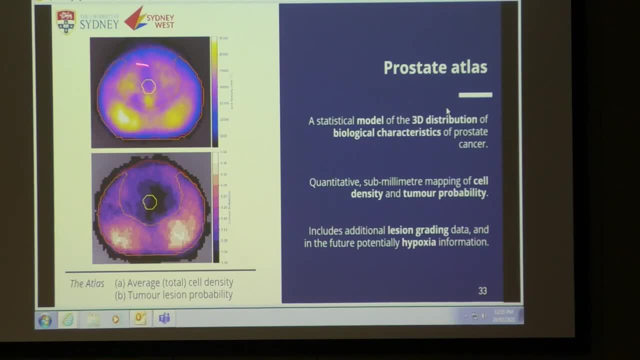 get our maps of the prostate. So here's a map of the prostate atlas showing the total cell density and you can see there's some hot spots here in the peripheral zone and a bit under the urethra. And here's a map of tumor probability. so where tumors occur in our 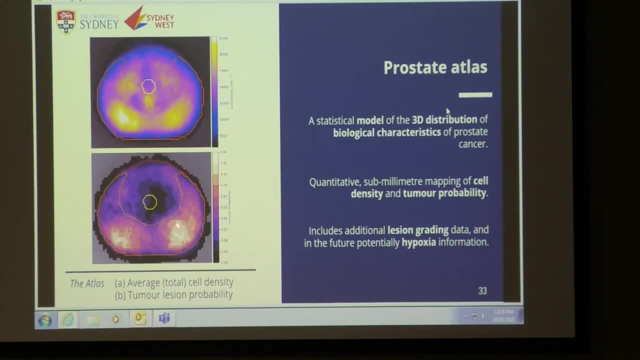 study population, where it's maximized in the peripheral zone. This has been known for quite some time. Prostate patients quite often get biopsies, and so you know that data is available to understand where tumors occur. but now we're looking at it from a different way. This 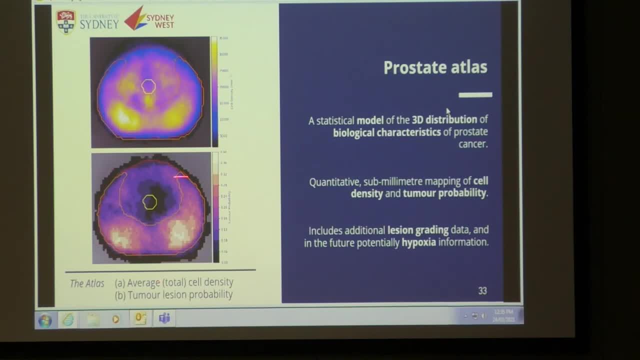 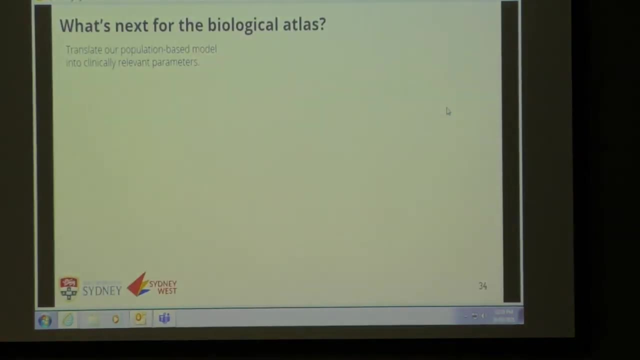 all includes additional lesion grading data. so here's just a map for every single tumor lesion, but we can break that down further into different Gleason grades, which is important to consider during model development. In the future, we also hope to include hypoxia information in this. So what's next? We 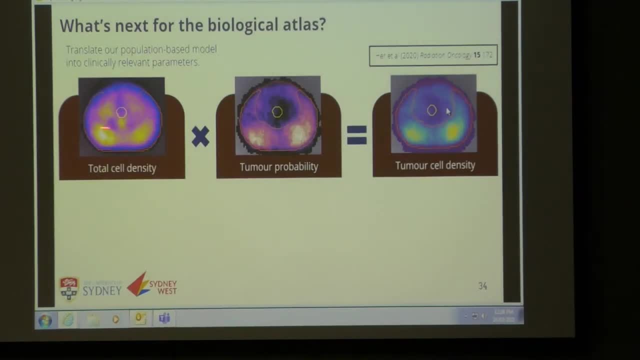 can use relatively simple mathematics. just multiplying these two atlases together- the total cell density and the tumor probability- to get an estimation of the tumor cell density. and this is relevant to optimize the TCP, for biologically optimized radiotherapy. To go even one step further, we can start to look at variability in the input. so 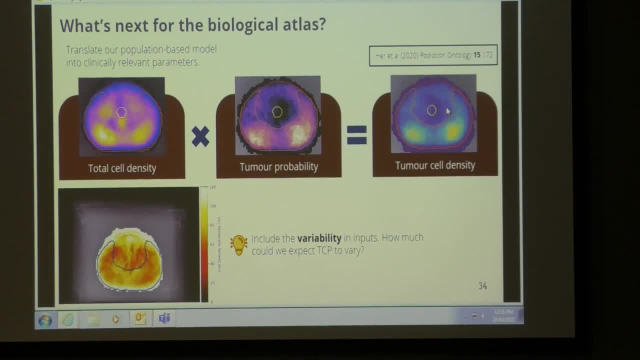 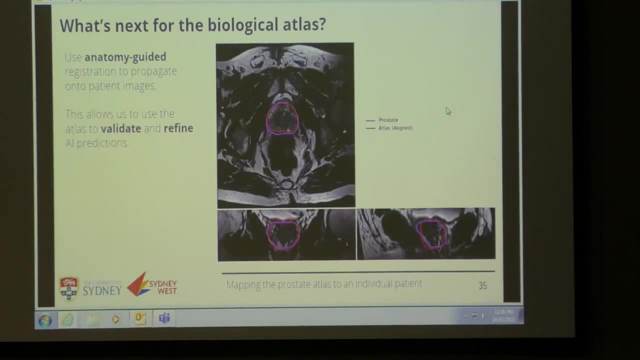 variability in cell density, as I've shown here, which can impact variability in tumor cell density and variability in TCP. To refine these AI predictive models, we obviously have to map this atlas to a patient, again achieved using deformable image registration, which allows us to validate potential AI predictions and also refine them. You can see here this. 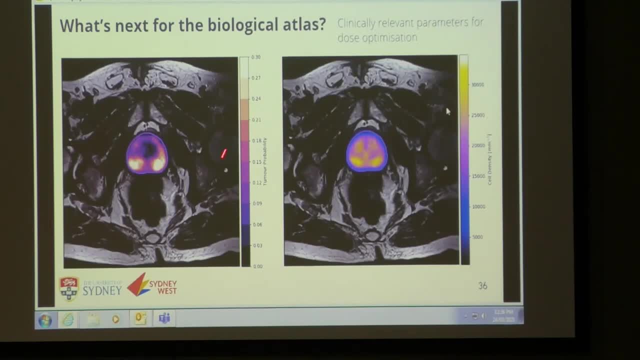 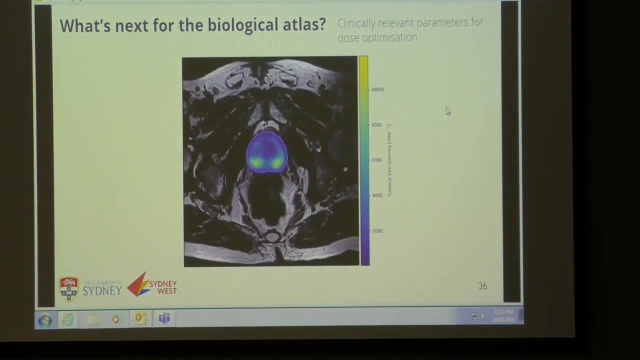 is just the atlas mapped onto an individual patient scan and we have a estimate of tumor probability before we use the AI models. and this is just the tumor cell density. We could also use this information as a sort of starting point to start to look at different treatment modalities you know like for on the population level. 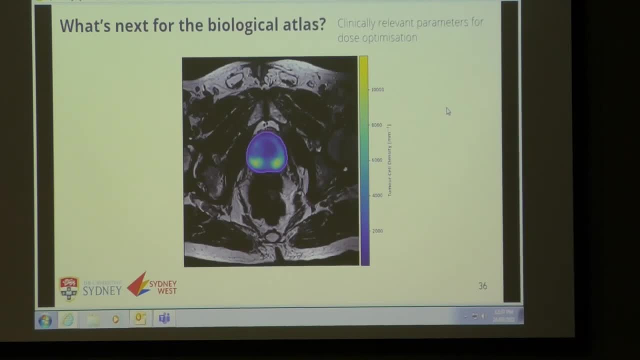 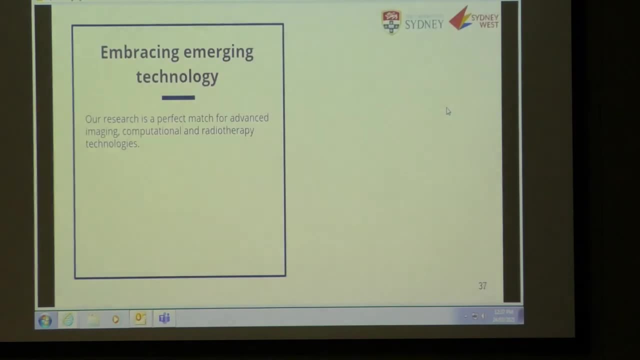 how can we use protons or cyber knife or, you know, brachytherapy, whatever, and we can use this model to actually generate that data. It also ties in well with the emerging surge of MR based radiotherapy. The MR LINAC is obviously becoming a more. 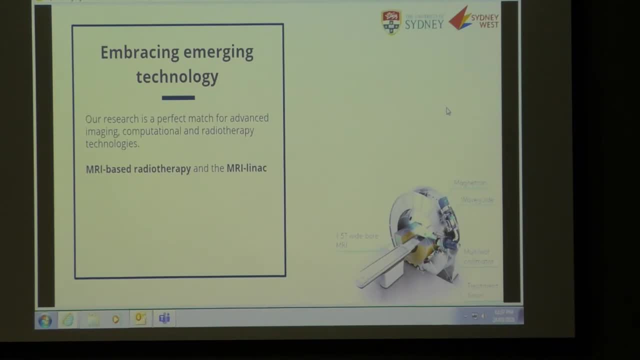 popular treatment modality- I think there's a few in Australia already- and if you can take a multi parametric MRI immediately to treatment, you can actually do this on the fly. you know biologically adaptive radiotherapy. The world of AI is, you know, making leaps and bounds every day and we hope to use as 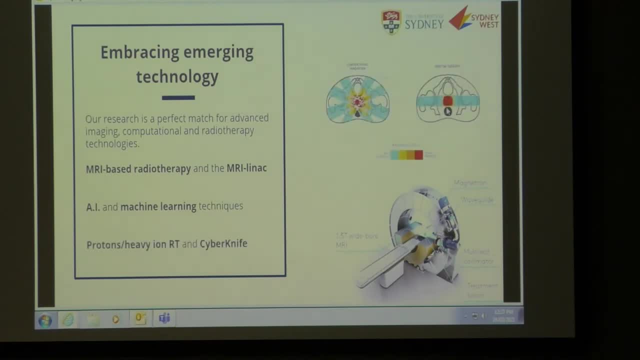 much of those tools as we can to improve this even further and, like I was saying, we can start to look at innovative treatment modalities like protons, heavy ions. we're getting our first treatment center in Adelaide, with another one potentially on the way for Westmead Hospital, and really we should start. 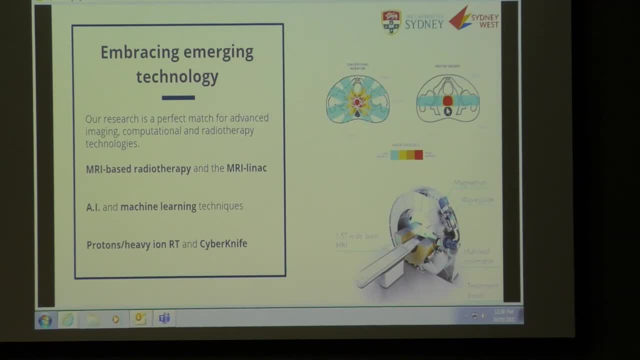 looking at moving beyond what we currently do not think about it as just more accurate radiotherapy. but, you know, adapting these treatments to really target the biology. You have a cyber knife here in Perth, you know, which can deliver extremely small stereotactic doses which could target individual. 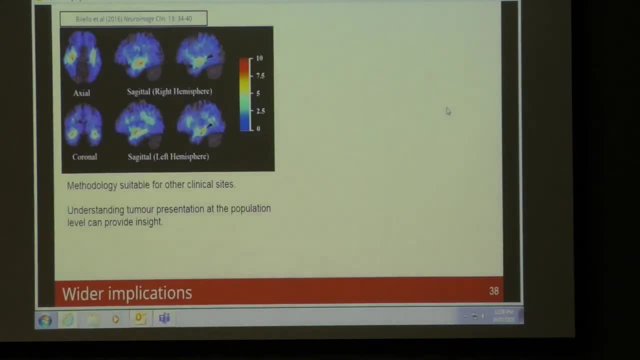 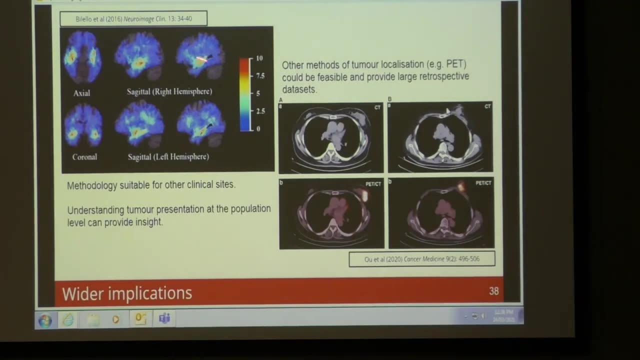 tumor lesions, potentially Some wider implications for this sort of biological Atlas based methodology. it could be applied to other clinical sites. some people have used it in brain imaging. I don't think this is to do with radiotherapy, but it might also be. 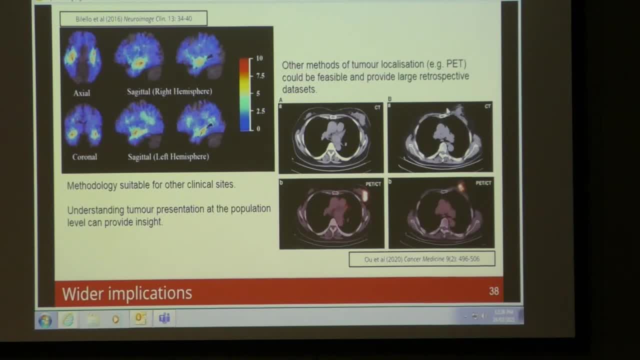 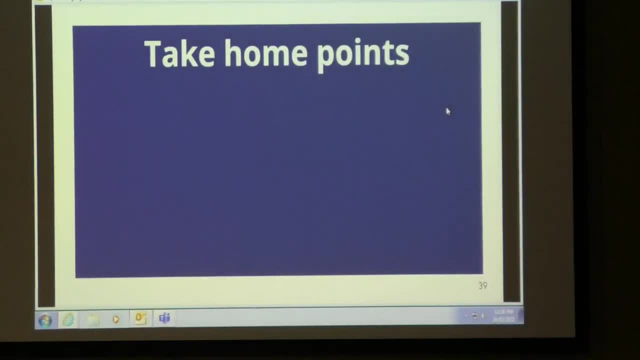 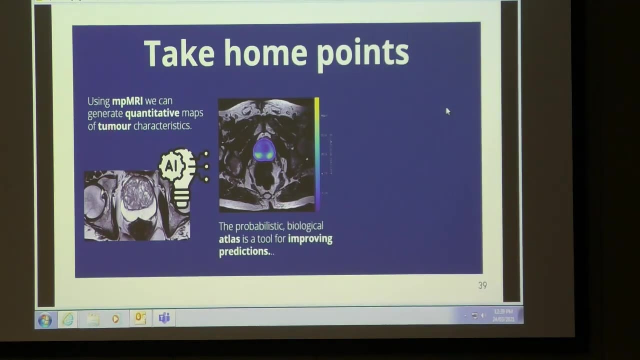 possible to use other methods of tumor localization, like PETCT or SPECT, to other nuclear medical scans. So multi parametric MRI is a really great tool. We can use it to get models of tissue characteristics, and the biological atlas is a tool that we can use to validate these predictions and also refine them. 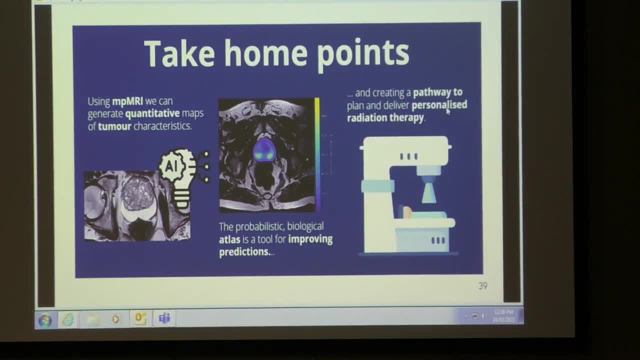 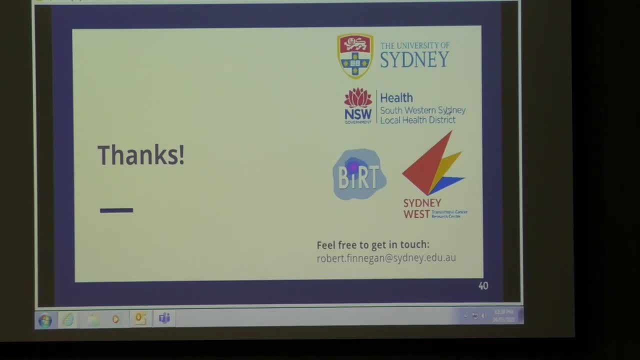 Which create. create a pathway to personalize biologically targeted radiotherapy. All right, that's all I've got, so thanks very much, and if you have any comments or questions, I Answered them all as I went. that's good, Yeah, Yeah, I think it'd be interesting also. 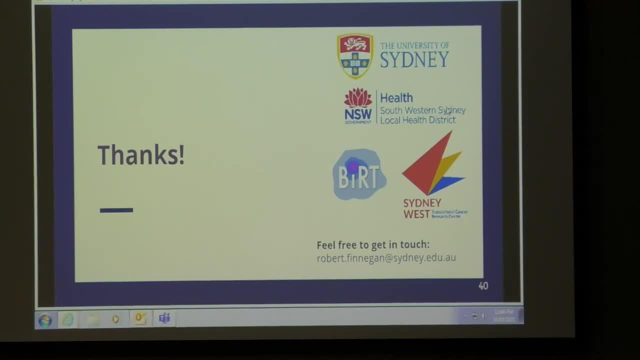 So the flame study was a dose escalation to dominant lesion. I wonder how that would tie in with dose reduction to areas that we can predict of not containing tumors. You know, that's sort of the next step as well. What was that sorry? There is a lot of uncertainty. there's uncertainty in every process along the way and, as you saw, there's a lot of processes along the way. 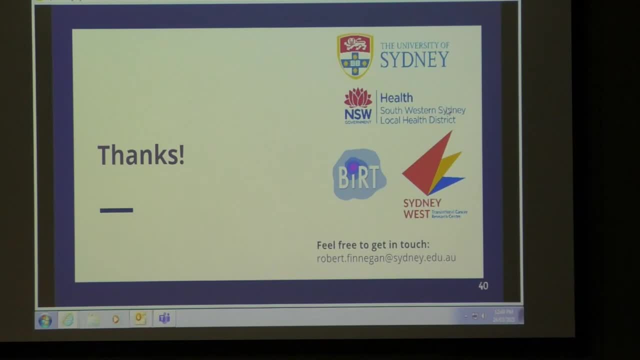 so in terms of like spatial uncertainty of the Registration, that's on the order of three millimeters. So predictions that we can make probably around that level. in terms of the uncertainty in the maps of the biological characteristics, We can actually quantify them at the out of finer level than just an overall like 10% or something like that.